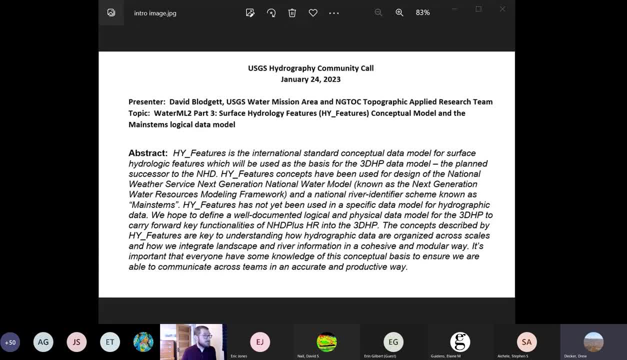 What we typically do with each call is go ahead and open it up, ready announcements from the hydrography program leads, and today what we'll do is- I'm going to turn this over to Steve Hale, who's one of our three program leads. who's going to introduce? 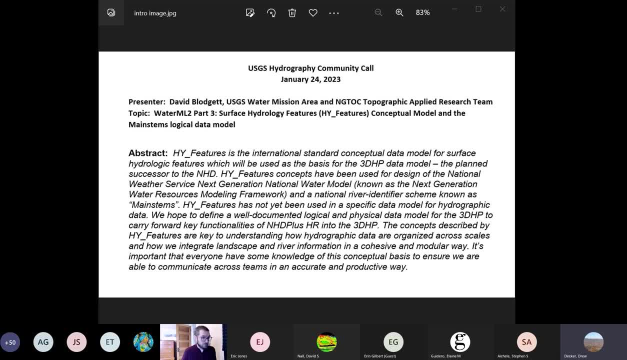 David Blockett, who's our speaker today, And before I turn it over to Steve, I want to mention what we'll do is we'll have the intro, we'll have David's presentation, we'll have some time, hopefully, for a few questions and answers. 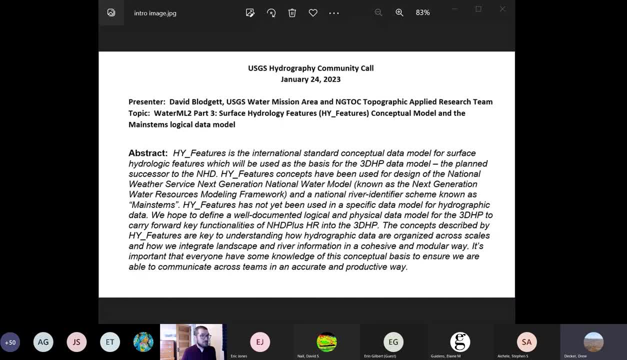 And then we can also open this up for any hydrography-related announcements from the group, and by the group I mean anybody on the call. So that's typically what we'll do, and then we'll close and I'll provide a little info on the date of the next call. 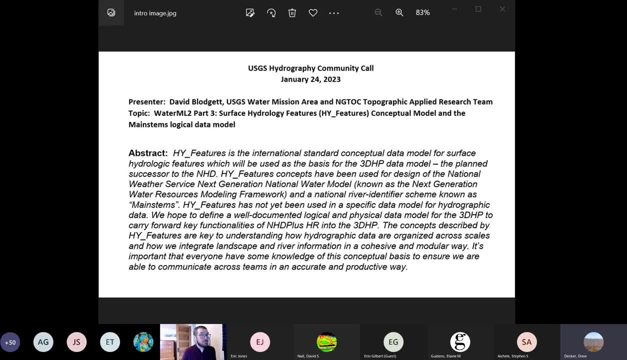 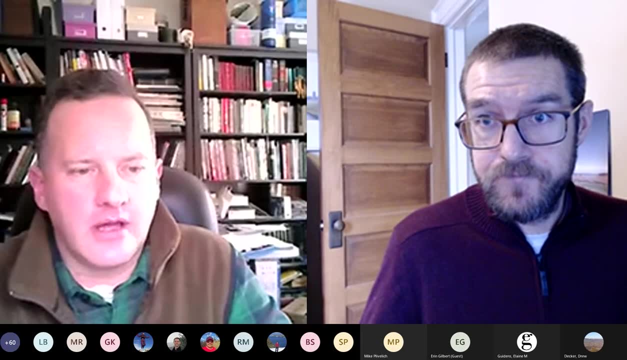 So, Steve, would you like to take it away? I'll stop sharing, Sure. Thank you, Drew. Thank you All right, So I guess, first off, I'd like to thank everyone, particularly all the folks that have been closing up your editing jobs. 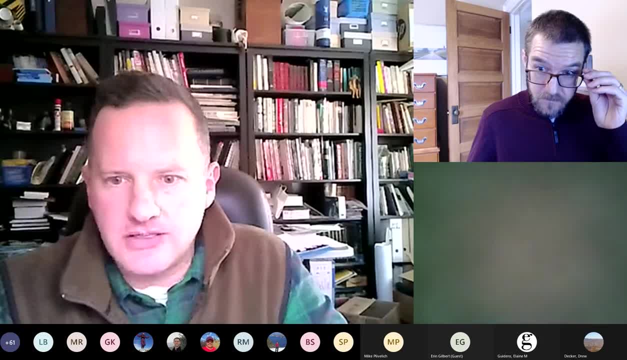 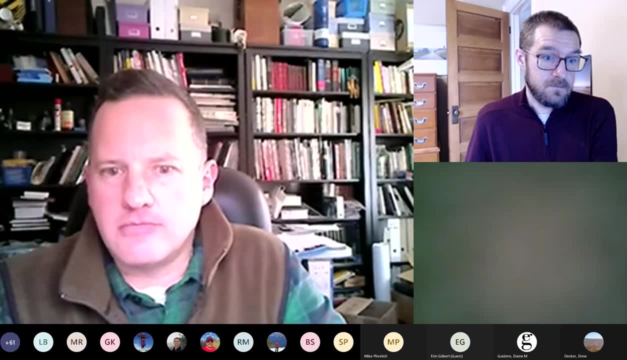 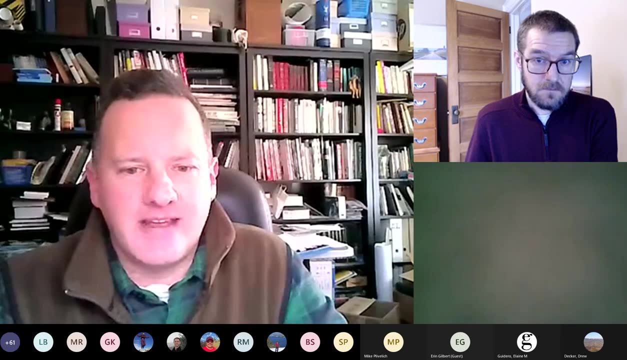 and we've got a lot of good markups into the system. Those are getting worked even now But we're making progress on winding down NHD As we go forward. we've been at NHD for 20-odd years and we really need – we've approached NHD. 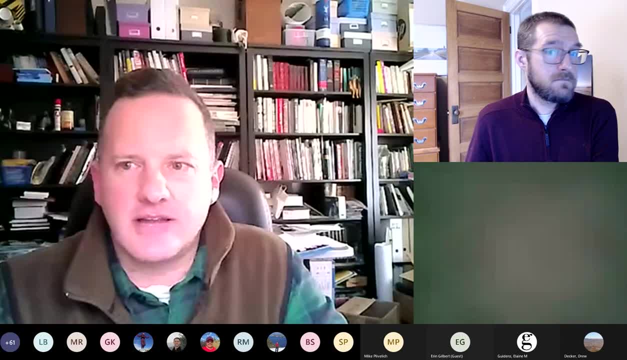 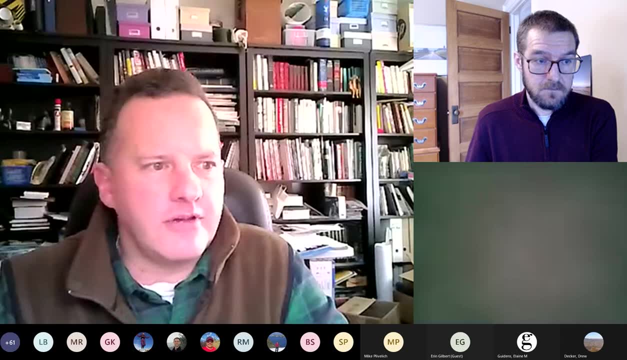 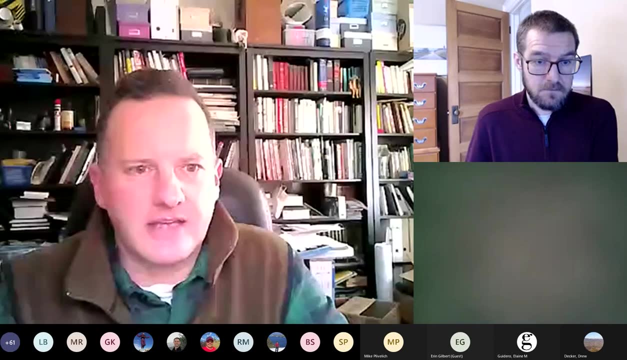 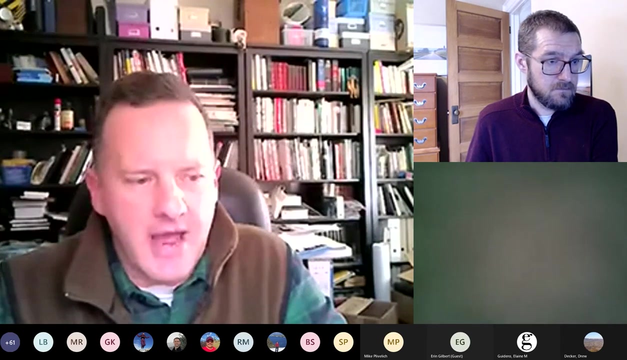 largely as a cartographic data set, as sort of representing hydrologic features on a map, And as we move into 3DHP we're transitioning that to really trying to represent hydrologic features as digital features, but as they exist in hydrology rather than as we'd represent them on a map. 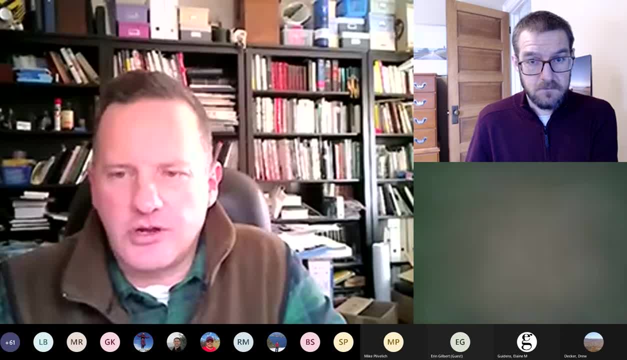 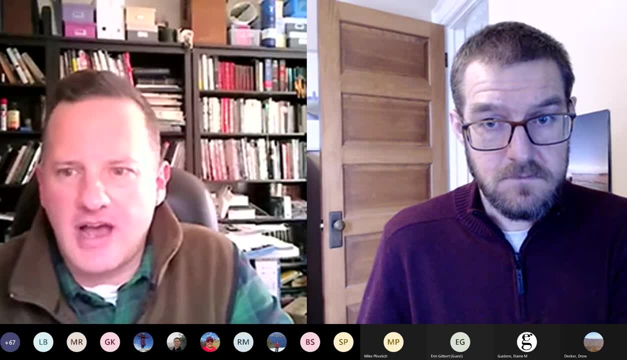 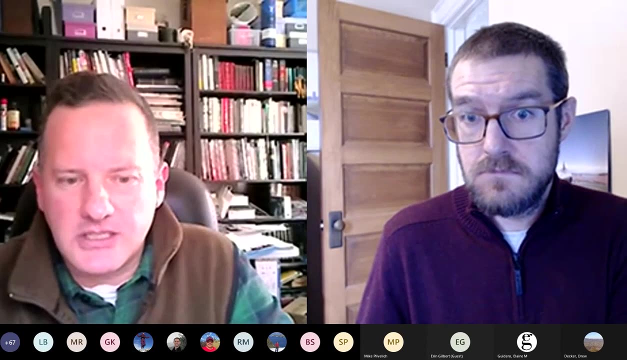 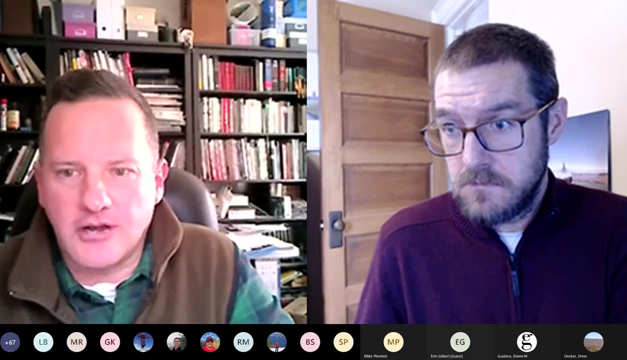 And part of that – I've mentioned this before on some of these calls It's transitioning away from the sort of classic NHD data set data structure to something based on high features and hydrologic features that OGC has put forward, And we've been fortunate to have Dave Blodgett come over from our water mission area. 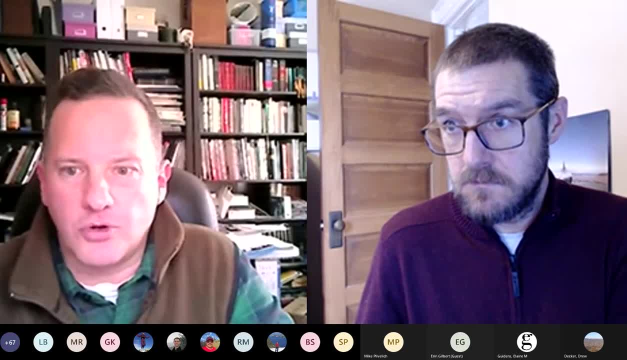 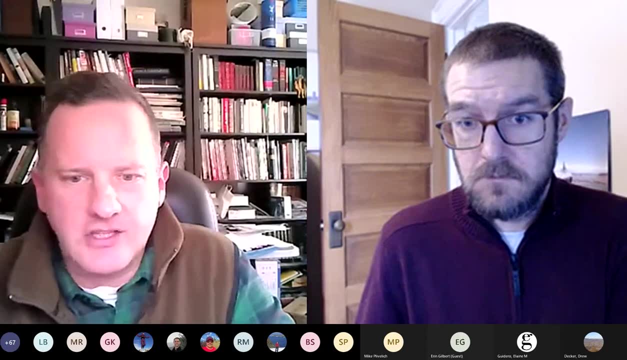 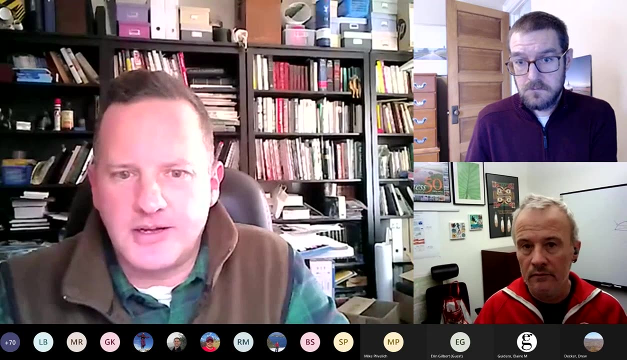 as the author of the high – almost literally wrote the book on high features to help assist us in making that transition, And so today he's going to do a little bit of a primer on high features from a high level And then, over a series of calls across the spring, here. 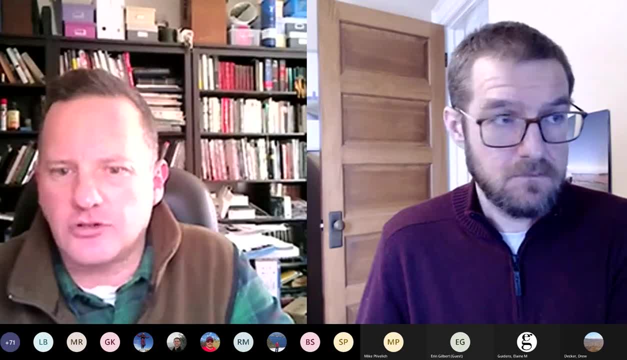 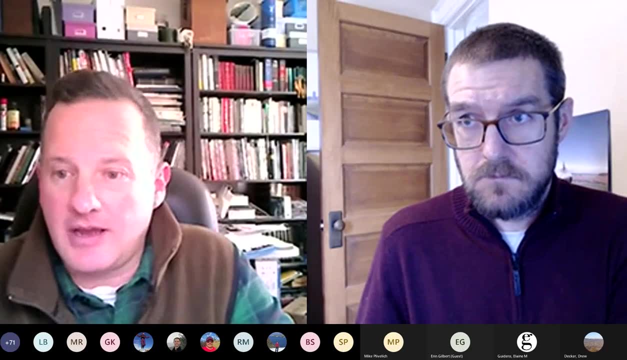 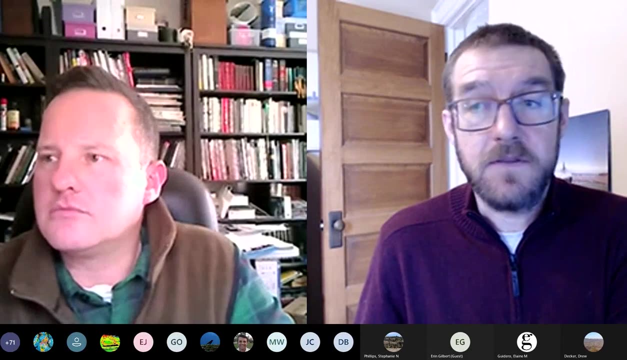 we'll gradually get more and more detailed into what that actually looks like in implementation, But today we're really just looking for the high-level concepts And I guess with that I'll turn it over to Dave, Dave Blodgett. Perfect, All right. So thank you, Steve, And 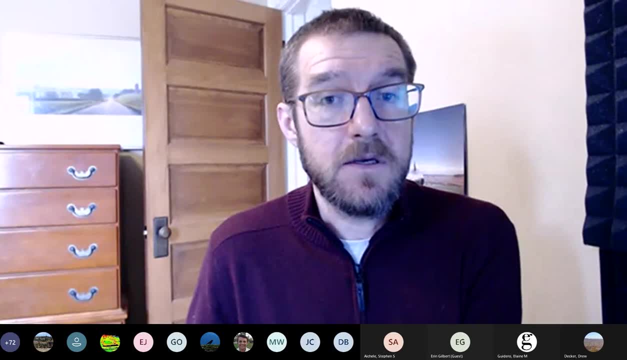 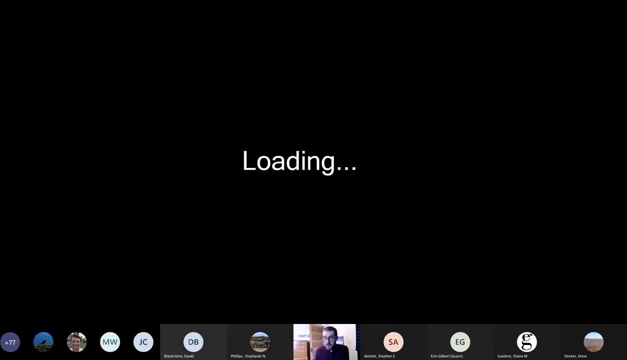 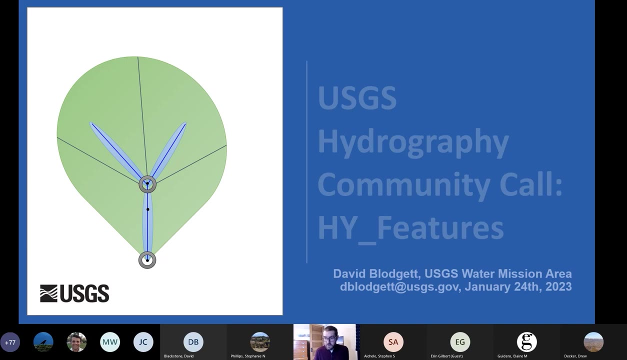 thank you for coming along everybody. This is a little different audience than I would usually interact with So I'm not entirely sure everybody's background and kind of prior experience and knowledge. But I'll do my best to make this relatable to what I understand this group's background to be. 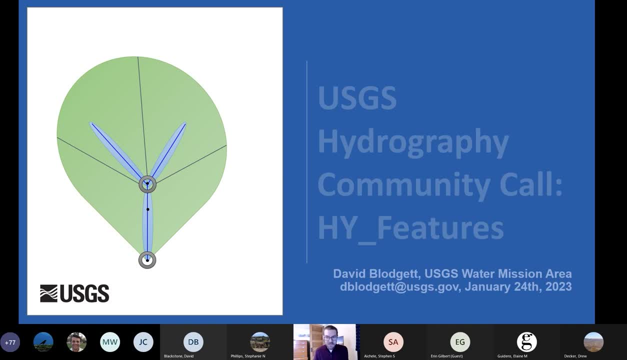 And so I've just put some slides on the screen using the Teams share, which will give you access to links, And you can move the slides on your own screen, I believe, if you want. So hopefully that works for everybody. 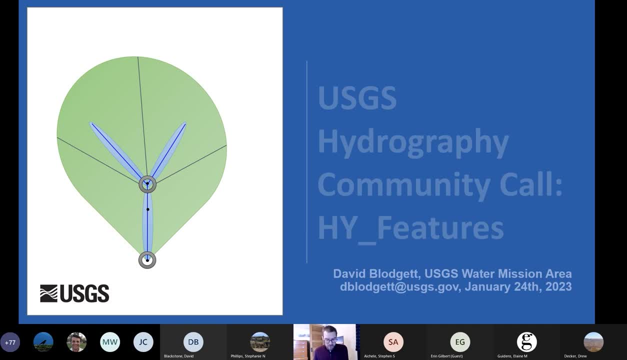 All right, So I'm Dave Blodgett. Came through the USGS's Wisconsin Water Science Center- Upper Midwest Water Science Center- now, And six or so years ago the unit I was part of became part of headquarters And I'm now in an integrated modeling and prediction division within the water mission area. 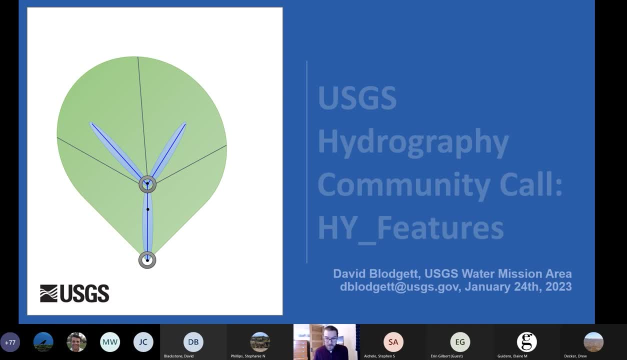 and sit in a geospatial intelligence branch And I describe myself as a hydroinformatics coordinator for the USGS. I'm an edge civil engineer, so kind of a research engineer with the USGS water folk, Dave Blodgett And I've done. 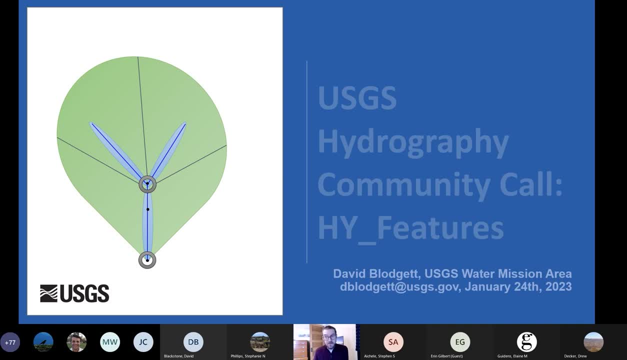 some different details around. I worked at the National Water Center thinking about the design for the next phase of the national water model, And now I'm on a detail with the National Geospatial Tech and Collaboration Center thinking about the future of NHD and 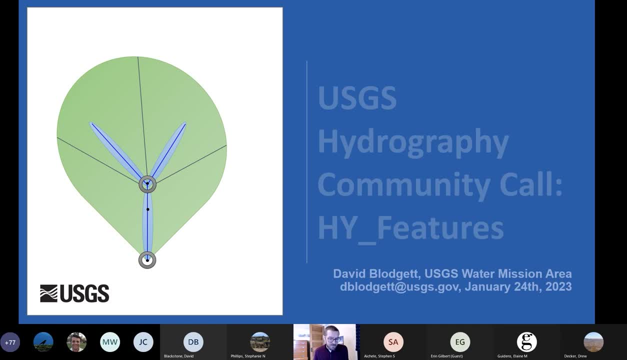 this 3D hydrography program. And so several years ago I was sitting in a meeting and this topic of high features was on the docket in the Open Geospatial Consortium, World Meteorological Organization kind of joint working group for hydrology. And David Maidment from the back. 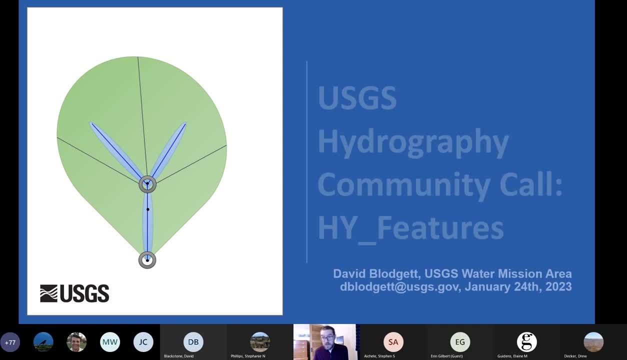 of the room voluntold me to chair the standards working group for hydrologic features. So I like to blame David Maidment for things, and I absolutely blame him for this being part of my portfolio, because I would not have put my hand up to do this if he hadn't suggested it. 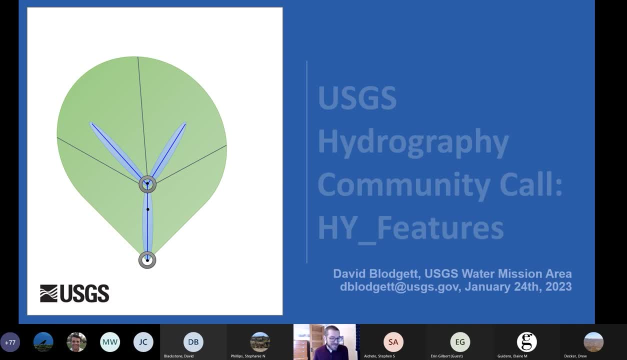 David Maidment. So the rest is history, And it's been quite a ride. This work came from kind of the brainchild of a person named Rob Atkinson, formerly of the CSIRO in Australia, and a woman named Irina Dornblut who worked for the Global 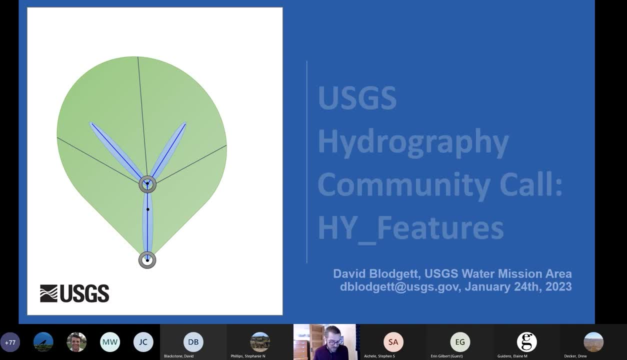 Runoff Data Center in Germany And I came in to help the two of them bring this work to fruition and bring, you know, bring the kind of the communication plan forward For this, this high features work. So there's just a little bit of kind of background and 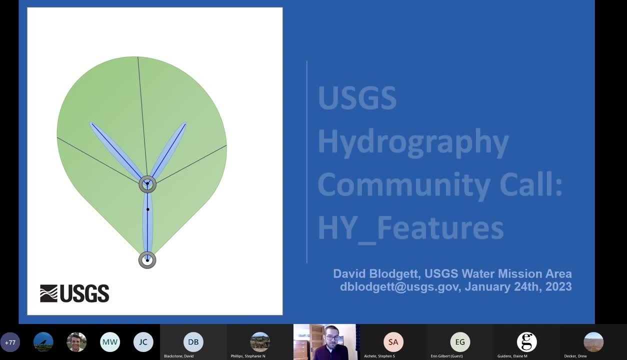 flavor of where this has all come from. It's it's based, this work is based on NHD, NHD+, the Canadian hydrographic model, Australian INSPIRE, so EU that it's based on and grew out of all these kind of global, continental scale hydrographic data models. but 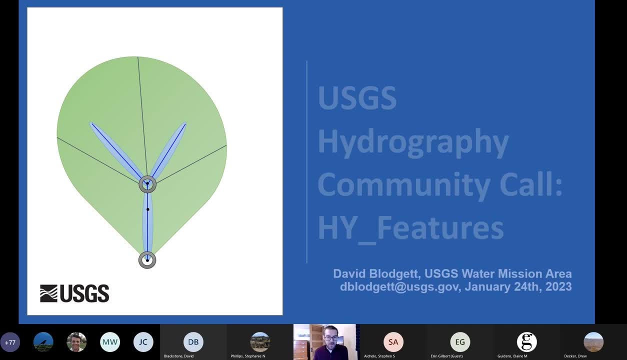 comes at it with a hydrologic lens, David Maidment, And, and you know it's, it's, it's, it's, it's, it's, puts kind of hydrology first And and so from a, from a modeling point of view, that's. 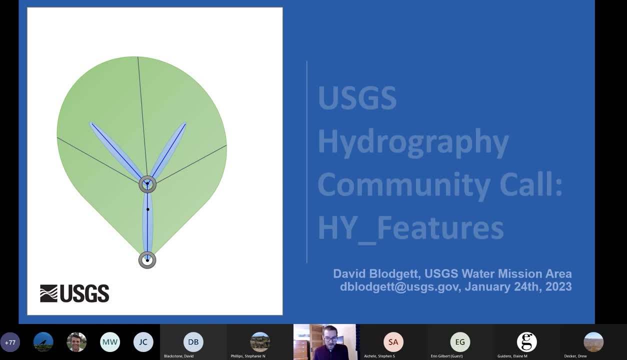 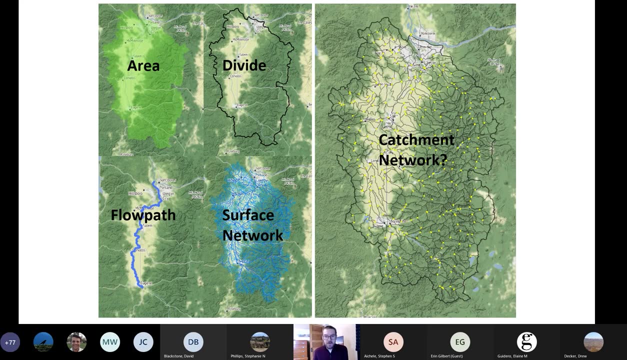 that's critical because- and I'll get into what that means. So that's enough intro, Let's, let's jump in. So at its core, HY features, or surface hydrology features. conceptual model breaks things apart in a in a fairly logical way, And I I wrote: 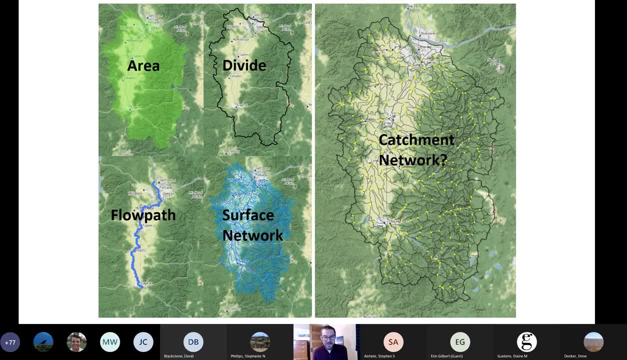 a while ago I wrote a, an upgoer challenge, which some of you may be familiar with, but it's a- basically describe a complex topic using the top, the, the, the top 10,, 100 or thousand. 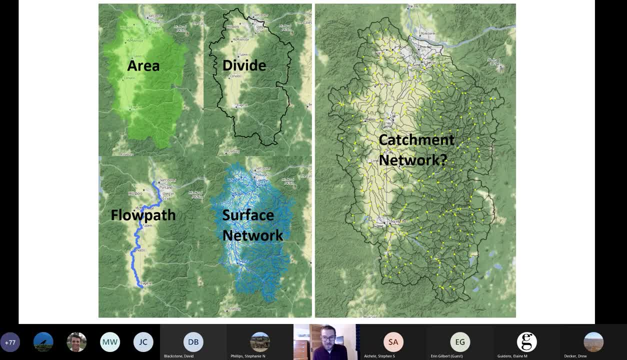 if you're going to use arcane- arcane words that people don't typically use. So, using the top 10, 100 words in the English vocabulary, And so you can go online and look up the upgoer challenge, You can find these text editors that allow you to write. 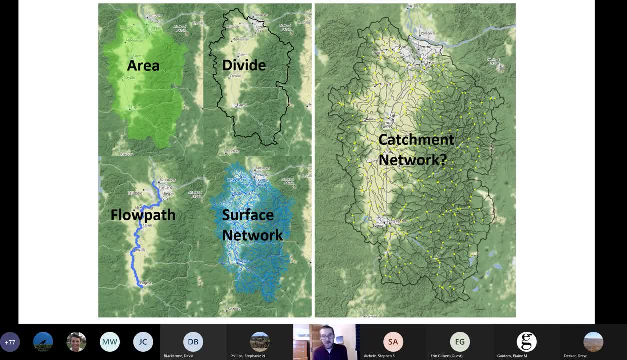 they they mark words that aren't in the top thousand words in the English vocabulary. So you you can write technical, technical descriptions using these basic common words. So I wrote that for HY features and I'm going to read it to you real quick. So I helped build a good way to 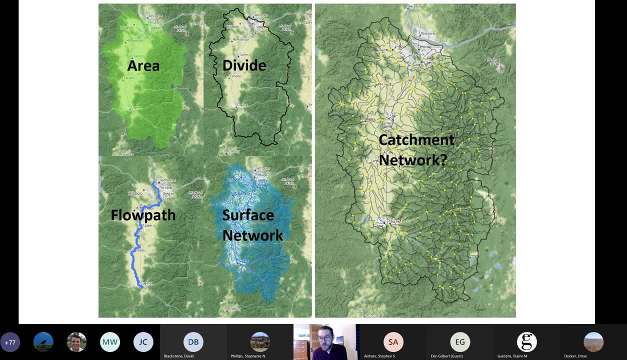 explain how we understand things in the world that catch water from the sky and, following in the down direction, group that water into bigger and bigger groups. We call these groups water bodies. The water catching things and their water bodies join and the water in them moves in the down direction. 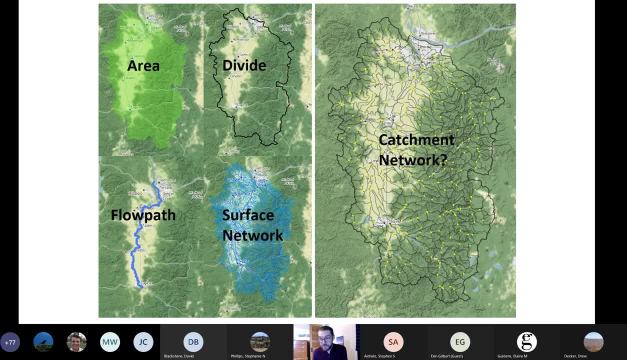 eventually getting to the deep blue water body. Although we think of a water catching thing as a single thing, we also think of the water catching thing as different kinds of parts that work together and form a whole. Some of the kinds of parts we decided to put in the good way to explain. 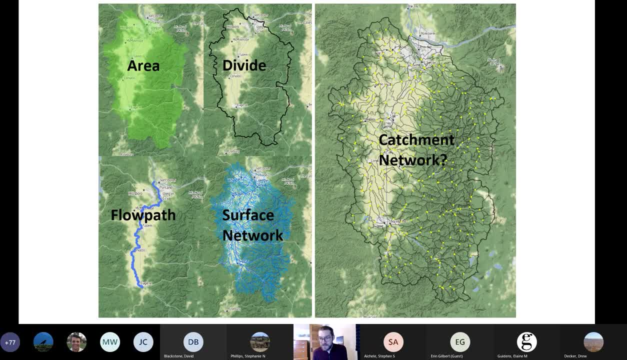 water catching things are its outer edge, the line water follows from its top to its bottom water. its inside area is like all its water bodies together and the water catching things that go with each water bodies. Each of these different kinds of parts is an important and special part. 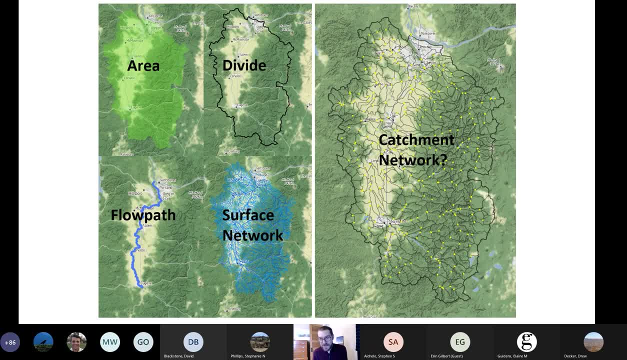 of the explanation of what a water catching thing is. Together they form the whole way to explain the water catching thing. Alright, so that just described the way. the inside of a catchment is the area, The drainage divide which goes around catchment, the flow path which gets water from the top of a catchment to the bottom. 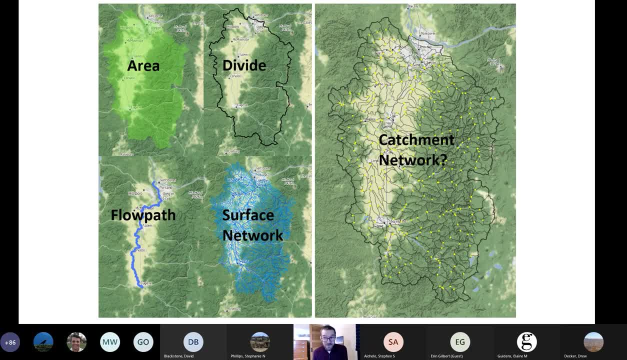 of a catchment: the surface network, which is the collection of water bodies that make up the network of water bodies within the catchment, and the catchment network itself, which is the collection of smaller catchments that nest within a given catchment. 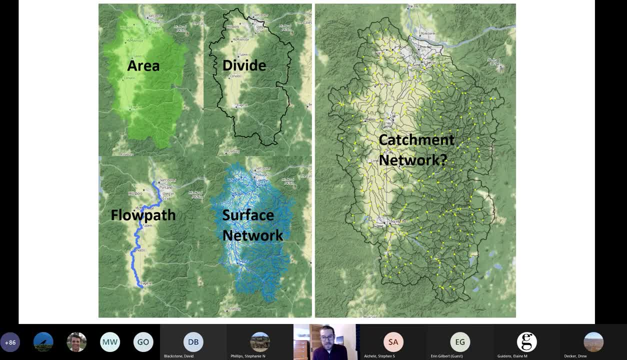 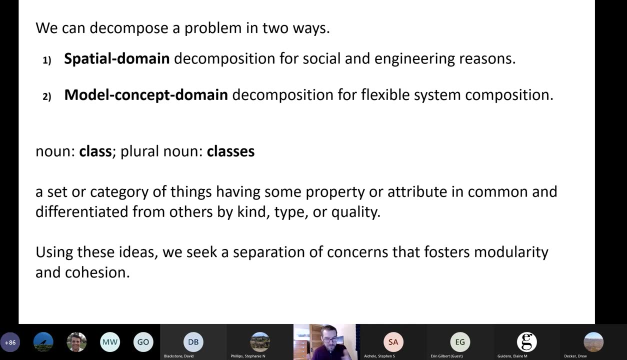 And this is the separation of concerns, and we'll get into that a little bit- that is defined by high features. It's these different kind of conceptual views or conceptual representations of this holistic thing we call a catchment, okay, So I've been alluding to this, I've been alluding to a few of these ways that we are decomposing. 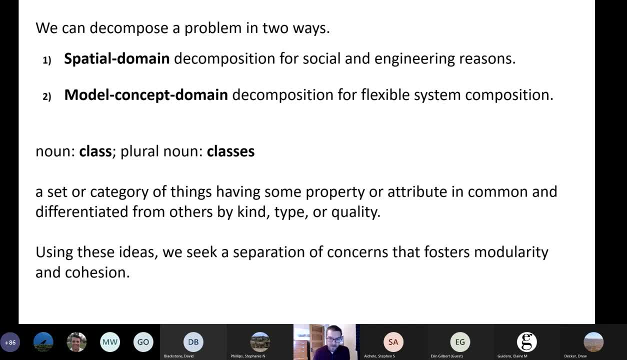 this problem in what I've talked about thus far. but getting into some very basic kind of specifics here- High features and this way that we're thinking about kind of this next phase of data modeling uses two ways, Two ways of decomposing the problem we're facing. 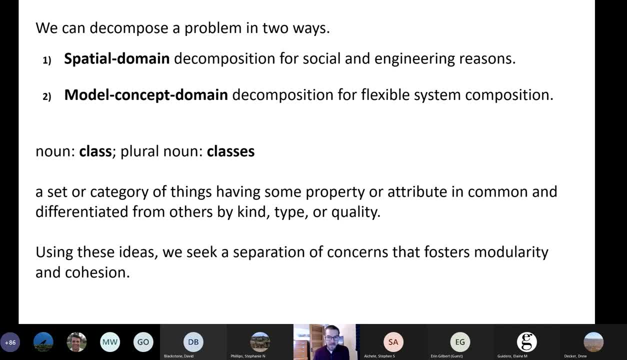 One is a spatial domain decomposition, the other is kind of a conceptual decomposition And that is like watersheds provide a really nice spatial decomposition of the landscape that happens to be networked right. It's a simple graph, it's a tree of connected landscapes. 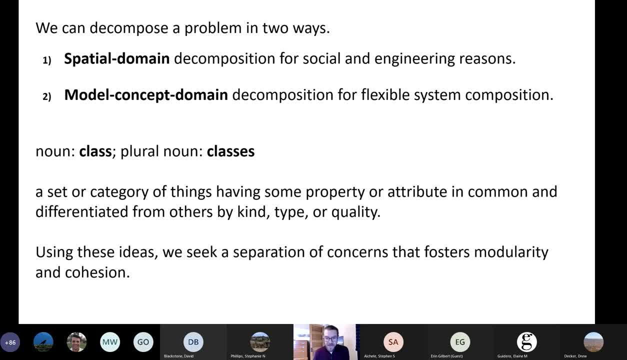 And then in the conceptual domain that's the area, divide, drainage, network, right, They're different conceptual representations. They're different conceptual representations of a watershed, ostensibly a catchment, And so those two ways of decomposing the problem are really important, just to recognize that. 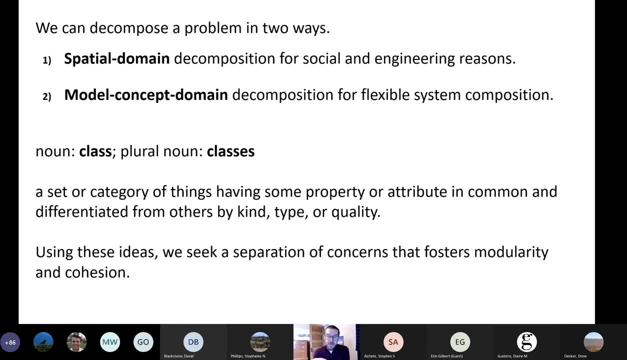 that's the tool we're using, And then this is a data model relying on this concept of class, And so a class is, in this context, a set or category of things having some property or attribute in common and differentiated from others by kind, type or quality. 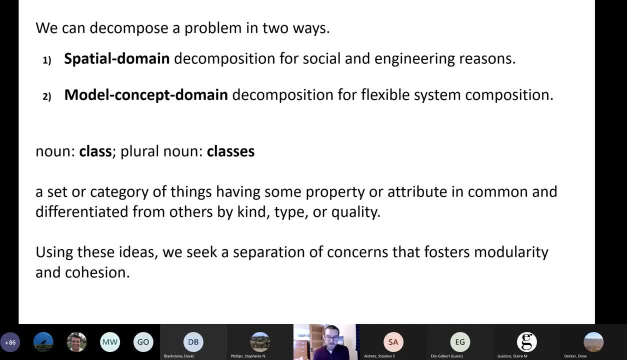 And that's also pretty straightforward, but also very important to remember that the precision, so the abstract, the abstract basic terminology that we're using here Needs to be heard through a lens of class, and that these words imply that these things are different from other things. 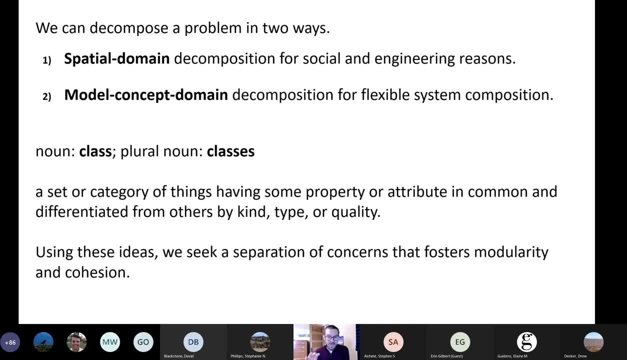 others by kind, type or quality, and so that we can't let ambiguities basically leak into how we're talking and describing these entities that we're building into our data sets, and that's very important. So, finally, you know we can use these. These are essentially the tools we're using. 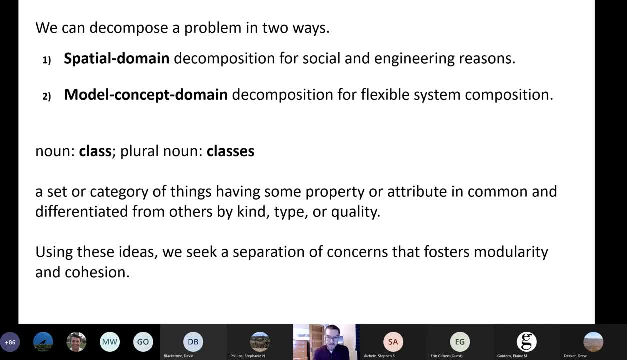 for a data model exercise in the hydrology domain, science domain, and we're using these ideas to seek a separation of concerns. that's fostering modularity and cohesion. and modularity being how well separated are the entities in your design, cohesion being how well do they work together? 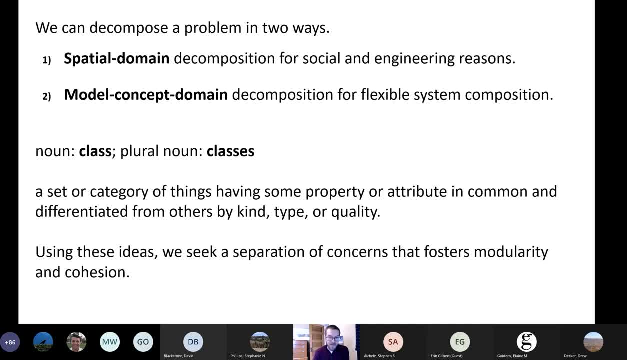 how well do they fit? how good is the interface between one thing and the next? right, And these are computer science concepts, but in kind of information management, data modeling. these are really important concepts to think about and get right, so So 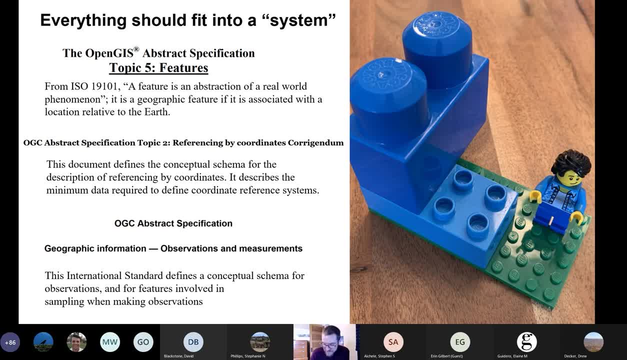 so I have a five-year-old and a two-year-old and so we play Duplos and Legos quite a bit. and, if you weren't aware, the Lego system is actually a multi-scale system. There's Lego at the lowest level, there's Duplo, and then there's whatever- these mega blocks or something. 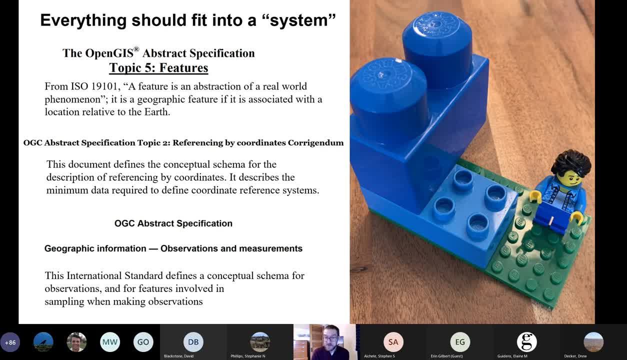 I don't even know what they're called. There are blocks that fit on top of Duplo and I think this is a really fun analogy for, like, even five-year-olds use a system that's actually pretty sophisticated and thought out and complex at the end of the day, Like Lord knows what you. 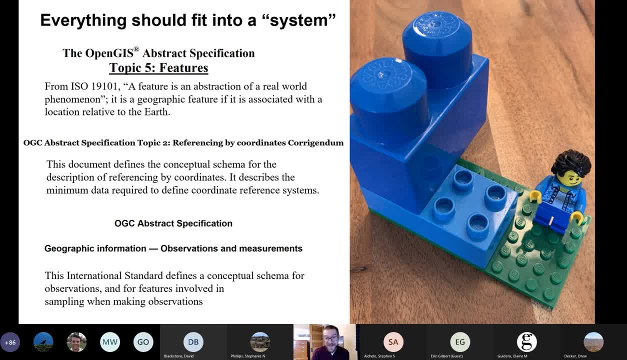 can build with a system of Legos and Duplos. People have built all kinds of crazy things that are way more complicated than most things we do from day to day, right. So the question is, though: what system are we using? What simple, somewhat elegant system do we use to build these? 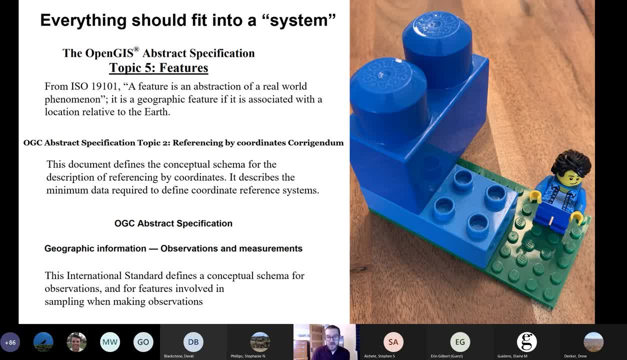 complex things we do in our day to day, And so there are some very basic building blocks here that we use to construct our systems, And so a couple that I have on the screen here that are worth being aware of this topic. five of the OpenJS abstract spec for features, basically stating a: 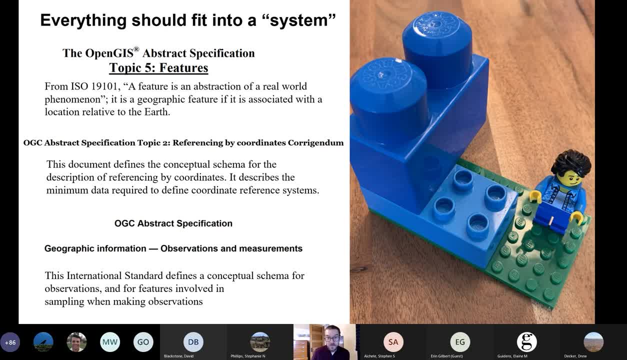 feature is an abstraction of a real-world phenomenon. that's fundamental. We represent digital artifacts right, And when they have a coordinate reference system and they have some spatial representation, they become geographic features, And so that's core to what we're doing. 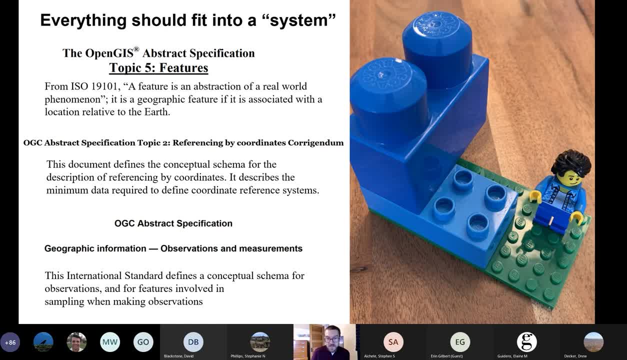 Then this next one: referencing by coordinates. right, That's kind of what I was alluding to, Like there's features that can be abstractly identified, say like a GNIS ID, but you have to give it a reference point, using referencing by coordinates, to actually make that a meaning. 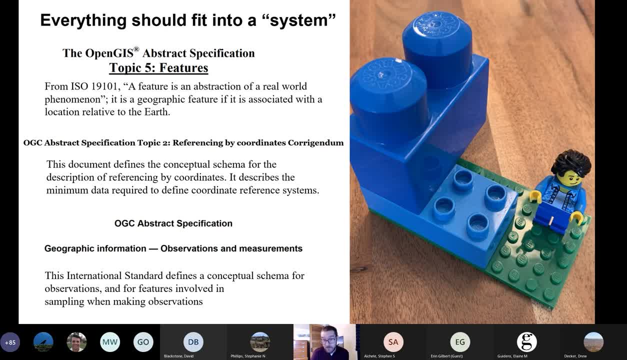 full piece of information to somebody who wants to look at it. right. You need a referencing by coordinates to make it into something you can put on a map. And then this last one: this idea of observations and measurements to people with a physics degree is actually a very 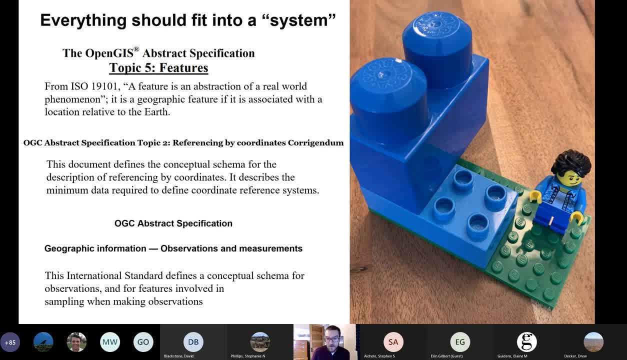 profound thing, because it's setting a standard for how we document the act of making an observation, And that's very important for hydrology, because what we do is make observations at locations along rivers that we can then use to make inferences about what's going on in the. 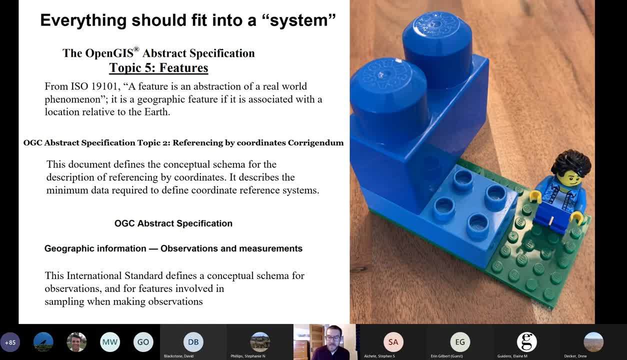 landscape upstream And the relationship between the observations that we make of phenomena in-stream have really important implications and really important relationships to a lot of things going on in that kind of broader context right, And so that relationship between observation, whether it's remote sensing or in situ, 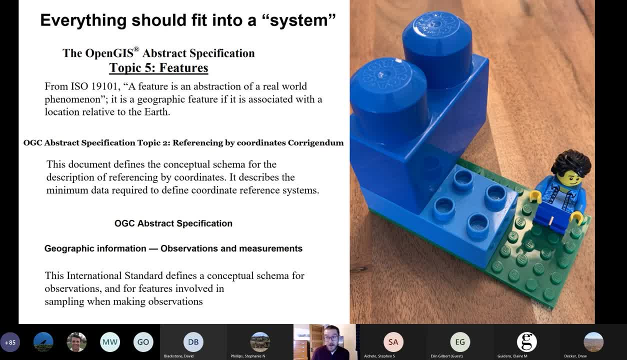 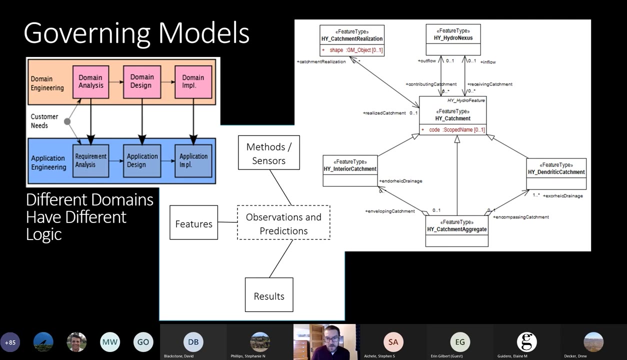 and hydrology, hydrography, hydrometry. these are all science domains that rely on this idea of observation constantly, And these are three key building blocks to all the information systems that we use in environmental science, hydrology, et cetera. Okay, so that's. I've got a little. 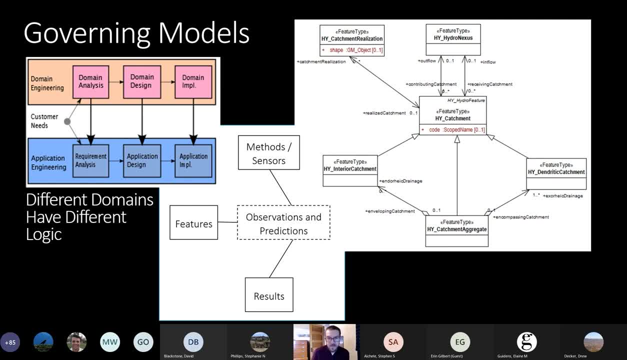 different perspective on these governing models and zooming in a little to a little bit more detail, The practice of using these data models in many cases is something that we would refer to as domain engineering, And that's where you have. let's go back. you have some common computing tools, right? 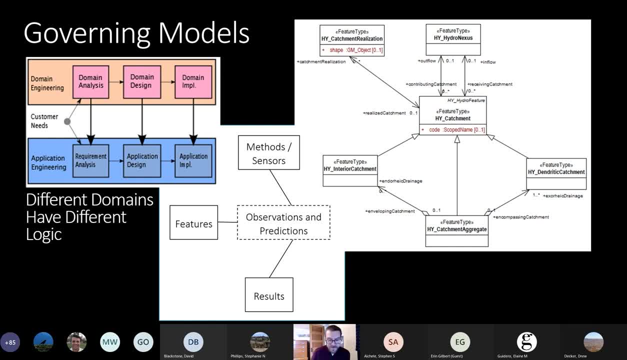 You have- I don't know- Excel and a collection of functions that you can put into cells in your Excel table. You use those application tools to solve problems that apply to a given domain problem. right, You always come. you always come to to your your computing tools with a specific problem. 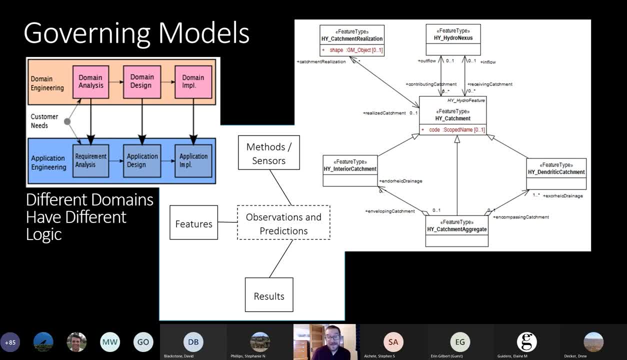 that's rooted in some specific domain of discourse, some science domain, right, And then you, you figure out ways to use these common tools to satisfy your customer needs, your domain requirements, And so this is a process that we all implement And it doesn't really matter. 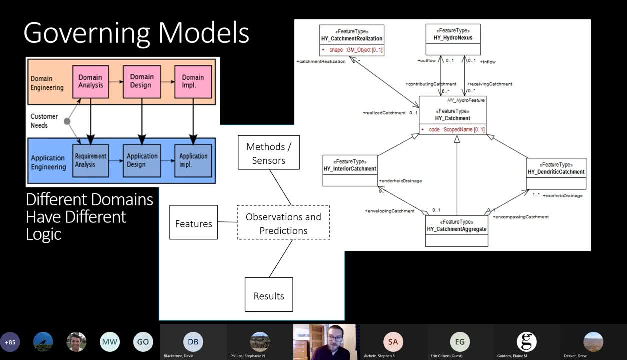 how sophisticated your tool chain is or how technically advanced you are. You're always using reusable general tools at some level to solve a specific domain problem, And we use these models to build increasingly nuanced tools that are still generally applicable across different people's specific problems, And so observations and measurements is one of the 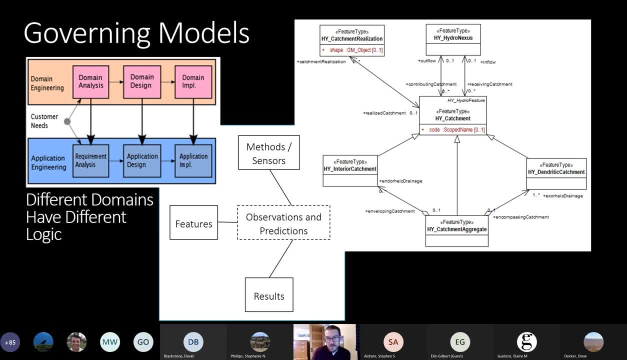 one of the tools that we do to do, we use to do that, And the reason I'm talking about observations and measurements here is the, the, the role of hydrographic features. hydrologic features is to give observations a reference feature So we can say I made an observation of that real world entity. 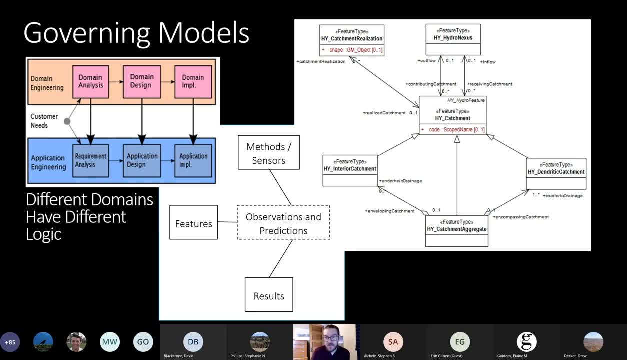 I made an observation of that river. I predicted the soil moisture in that catchment. I, you know. whatever it is right, You, you, you, you need to link a piece of information that's maybe useful for a decision process or something to the feature. 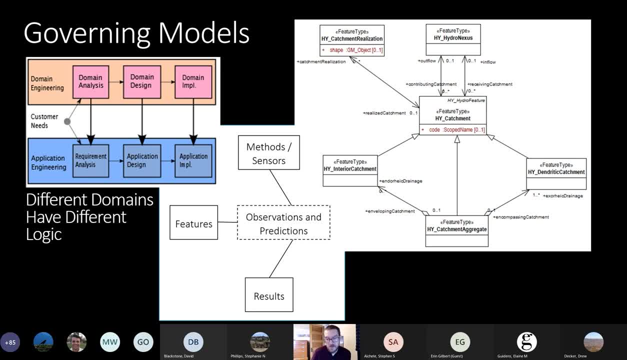 that it is actually bound to that makes it meaningful. Otherwise, it's just a number that's disconnected from from anything useful, right? So? so that's really this: observations and predictions. links to features. It also needs to link to methods, Sensor, what sensor was used. It also obviously needs to link to the actual number. that was the. 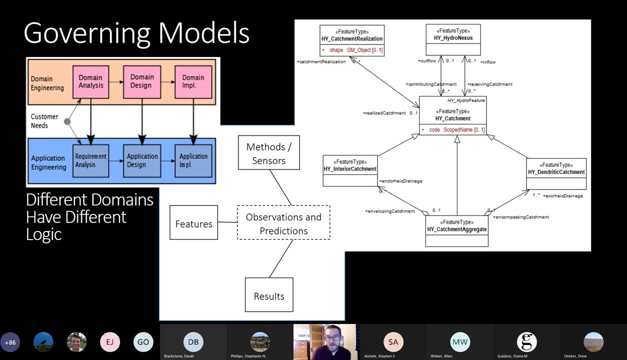 result of it. Um, but this is this observations and measurements thing that we we use and reuse for so many applications but don't really realize that this basic abstraction is kind of core to what we're doing. So that feeds over here to high features, which is, um taking this features box. 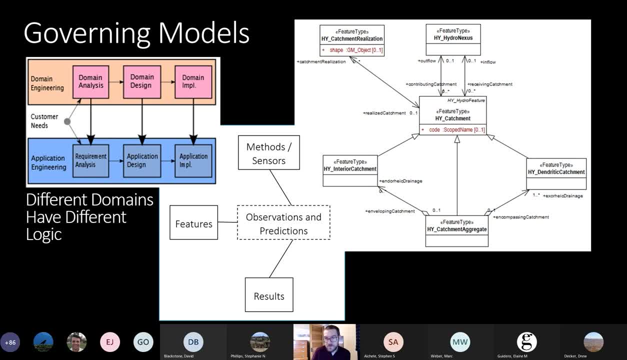 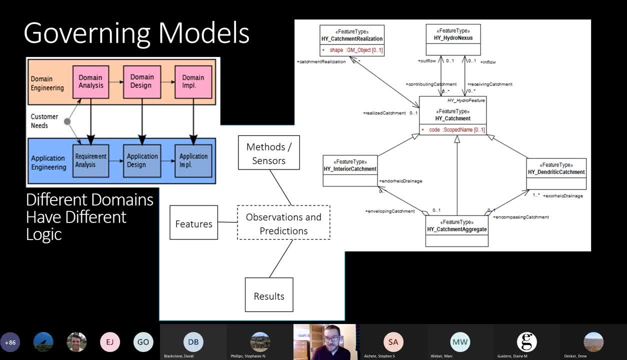 we have. catchments is units of the landscape that interact at nexus is so places where one catchment flows into the next Um, and they form multi-scale systems. They so catchments can aggregate into catchment aggregates, And those aggregates can be made up of either dendritic catchments, So once 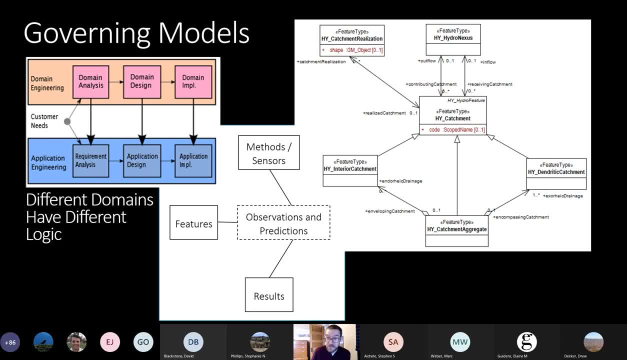 that behave nicely, like, say, watershed, boundary data set units um and interior catchments, catchments that that um don't flow out anywhere, right? And then there's this other, more complex form of catchment that might form. 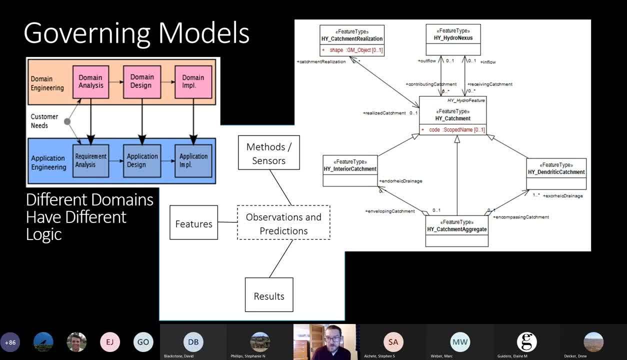 non-dendritic networks and that's just this generic catchment, right? So that's the core of high features. That's really at its base. it's just defining this ability to cross-scale with aggregation where no non-dendritic behavior exists, and this idea that catchments interact. 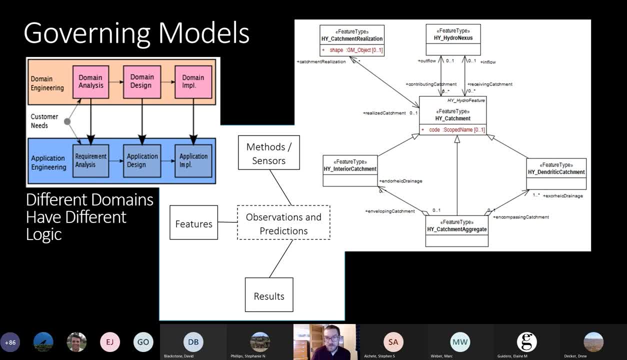 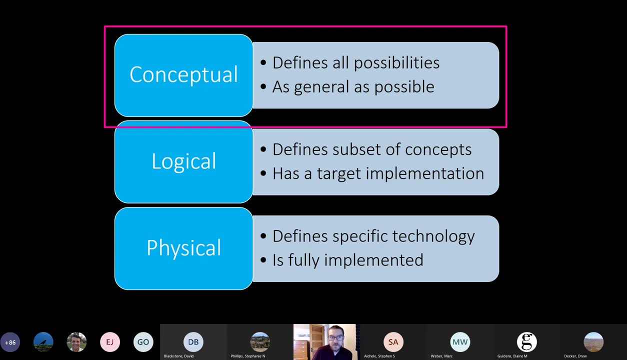 with each other at a nexus And then up here, this catchment realization is what I was talking about with my up-goer challenge. There are different conceptual representations of this holistic catchment feature. Okay, so another piece to- and this is all very basic and very 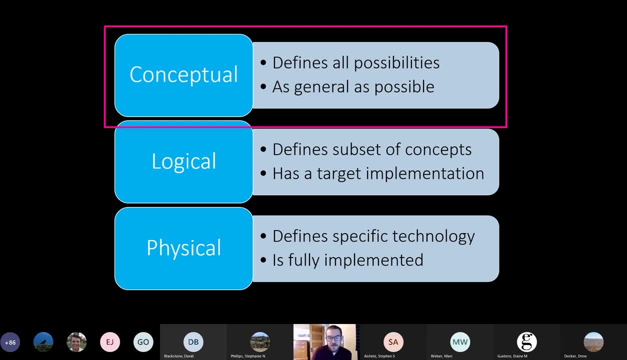 general. but the reason I'm starting here is high features, and this overall work is rooted in this level of generalization, so that we We can build things complex and have coherent building blocks to build from. so bear with me for two more seconds and we'll get to something specific. 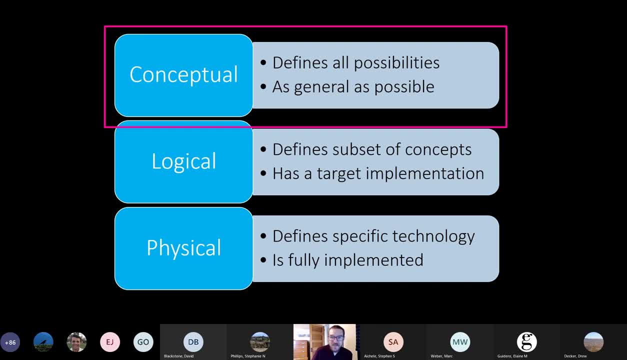 So the data model is defined in terms of concepts and the concepts define all possibilities and that is intentionally as general as possible. We're trying not to limit anybody in this conceptual space. We're just trying to nail down definitions, trying to nail down the potential. 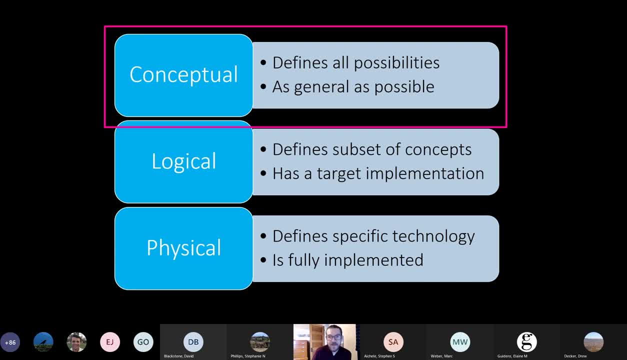 world of a conceptual space and we're just trying to nail down the potential world of a conceptual space. So we're trying to nail down the potential world of a conceptual space And then when we get into logic or logical representations of these concepts and physical 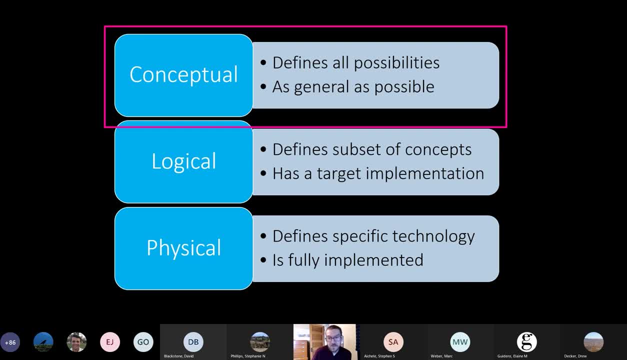 representations of these concepts. we get increasingly specific about constraints and the kind of specific business logic or specific domain semantics that need to be used to satisfy certain applications. And so back when I was talking about domain engineering here right a lot of times. 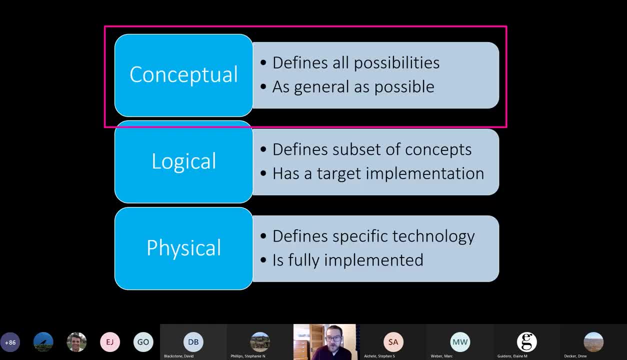 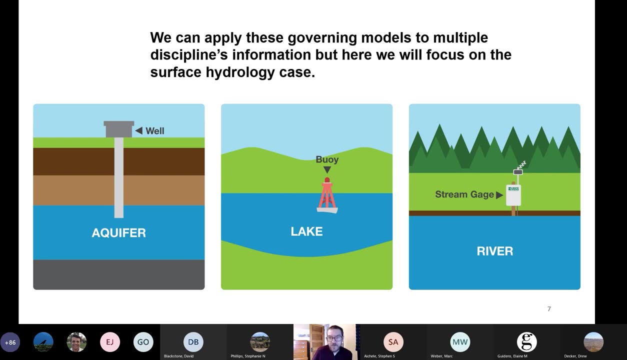 your domain, engineering process, is actually refining into a logical and physical representation of something that is much more flexible and probably overly flexible for what is actually needed. So okay, so now, getting down to earth, we can apply all these tools and governing models to our 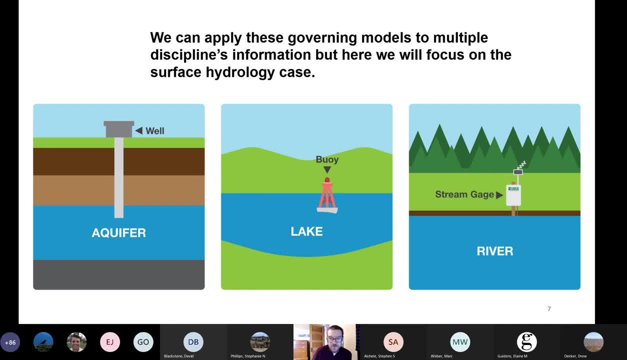 own applications, right. So we have features that are aquifers and we have monitoring features that are wells And we put sensors in them, or we go and, you know, drop some kind of measuring instrument down the well and we take observations and then we take that back and we feed it into a model and we figure out what's going on in the aquifer. 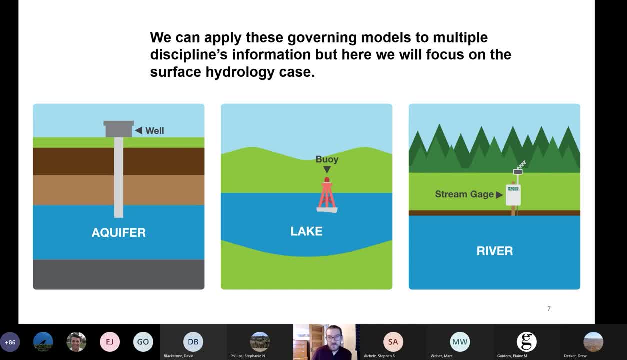 And we do the same basic: define a feature, observe it, make inference about it and then maybe predict things about it in lakes and in rivers, right, Right, And this. so this, this basic data model, holds up across at least these domains and it holds up across many others, right? 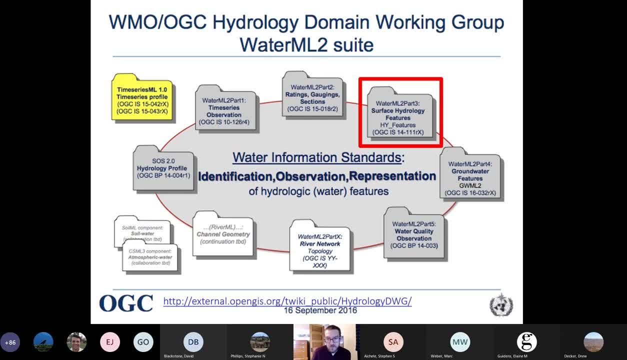 So I'm going to move a little bit well, so. so just a little more background on high features. that fits into a broader set of standards. So there's, there's one for the first one. part one was time series observations. 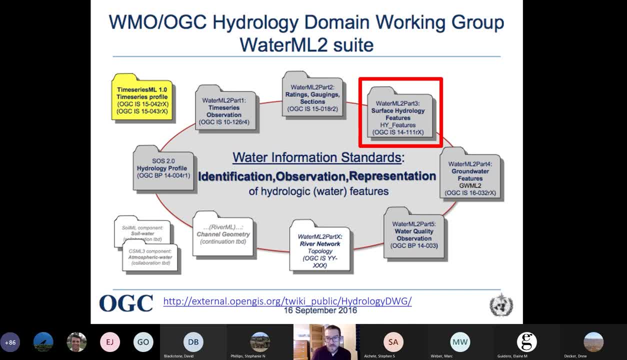 So stream, stream flow, you know, stage in a stage in a, well, et cetera. Part two is for ratings and gauging. ratings, gauging and sections, which is really. how do we measure stream flow as well, through a rating curve. 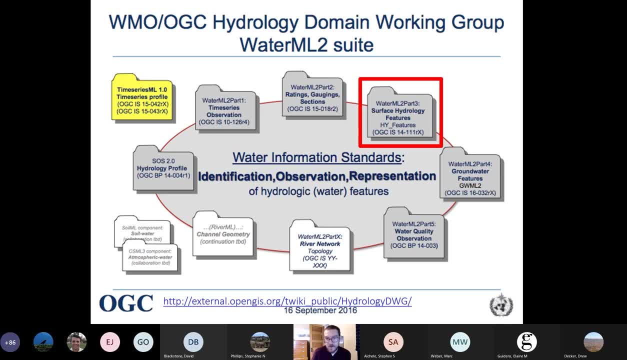 So we measure stage and we convert that into flow using a rating curve. And then part three is this surface hydrology features, which which outlines this set of feature types for hydrology. Part four is groundwater features. So same same concept but for hydrogeologic units and aquifers, and actually right now there's a interoperability experiment ongoing. 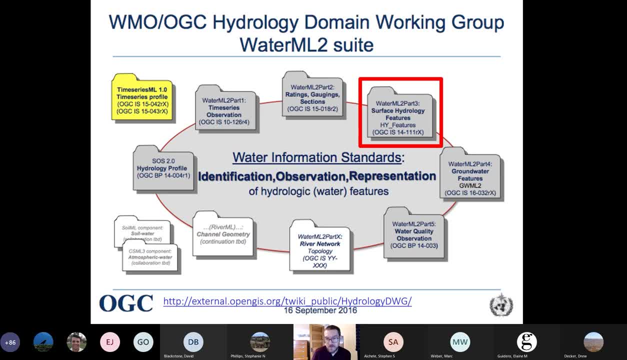 So y'all are going to advance this part five, which will be water quality observations. There's, there's more to be done here: River, river networks, channel geometry, water body representation, et cetera, et cetera. 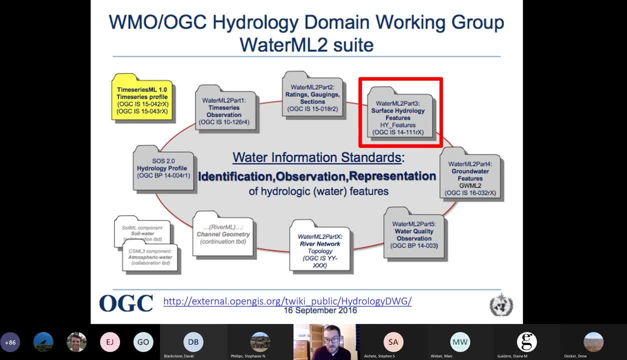 There's, there's a whole bunch more to be done here And it's it's a slow process. This is a this is a big international community process that's definitely gonna be slow moving And as this unfolds, you know, there the core of it is good. 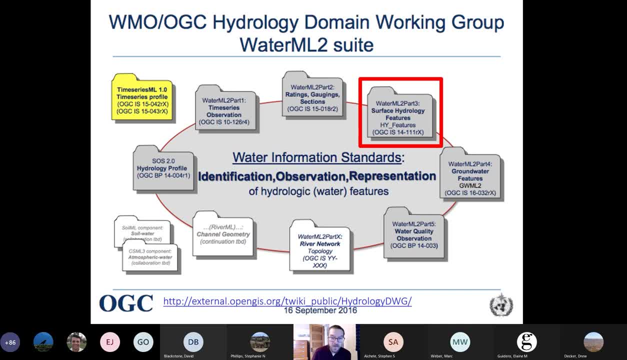 The core of it is built off the stuff that I just talked through And in. in general, it pays off for high quality, higher quality projects. we're going to see increasingly capable pieces and parts of this that become interoperable over time. 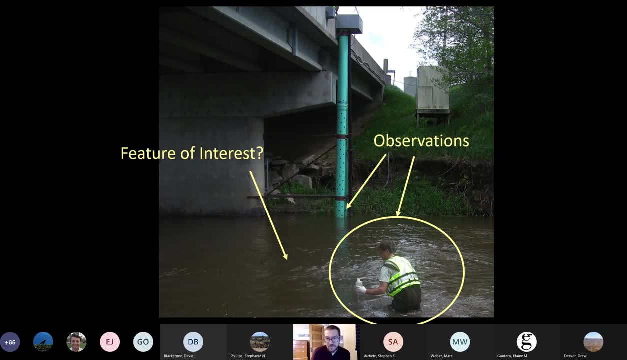 So let's dig into the hydrologic, hydrographic context a little bit here. So our feature of interest in terms of this, observations and measurements- is the river, And in this graphic we have two observations ongoing. right There's one in a stilling. well, where there's? 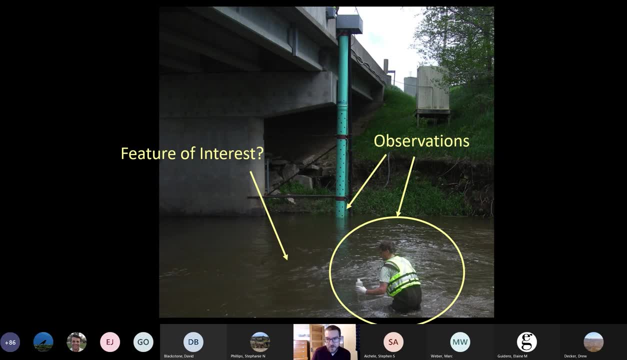 a sensor that's probably doing some temperature and stage, And then there's somebody in the river that's pulling a grab sample for some water quality measurement- probably right. So we've got two ongoing observations of one feature of interest And in high features terminology we have 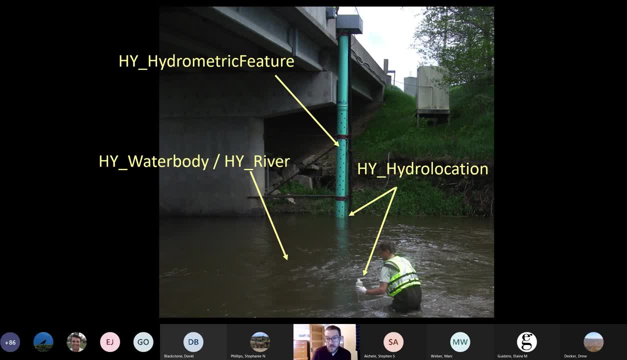 two hydro locations. One is the stilling well, One is where this grab sample is being taken. We have one hydrometric feature, So this we wouldn't necessarily call the person in the river with a bottle of a hydrometric feature. 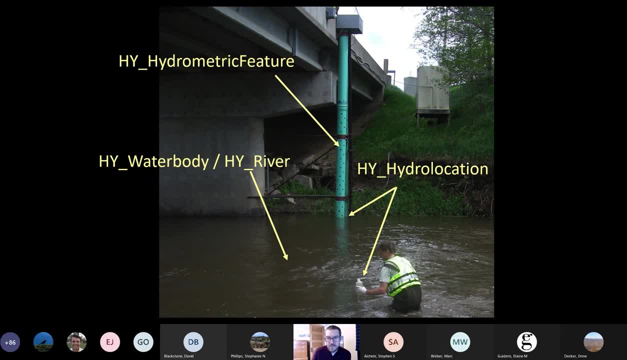 We would call this stilling. well, that's an installed piece of infrastructure, a hydrometric feature, a feature intended to support measuring hydrology, And then we've got this water body, which is of type river right. That's our feature of interest. So this is just digging. 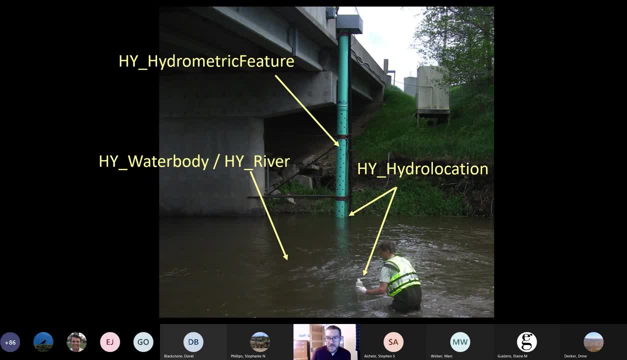 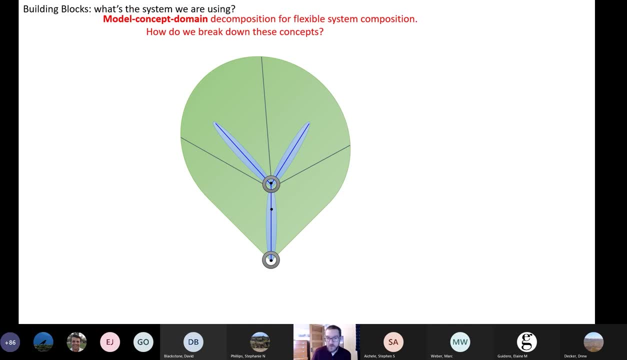 into some of the specifics of what high features would call this, And note that this is just taxonomy. This is just terms, Names, games- right, We're not really describing how they relate to each other yet. And so what are these building blocks? I have this kind of set of graphical representations of the way. 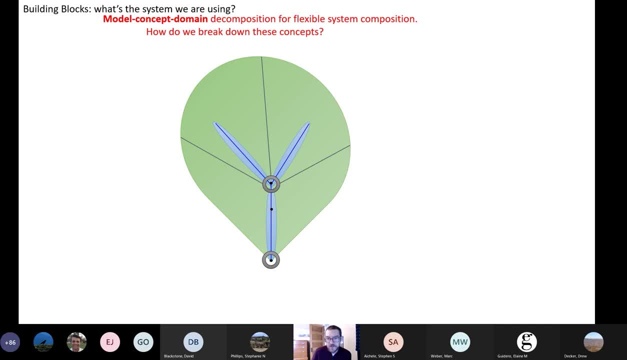 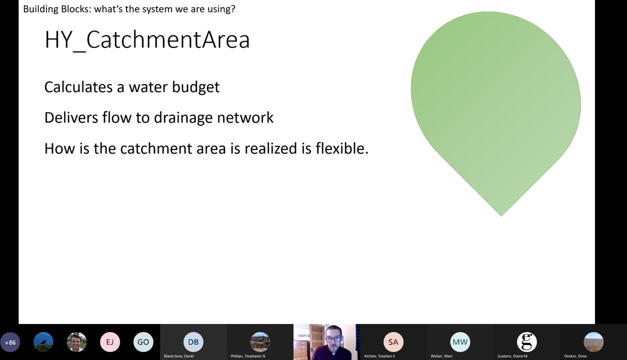 that we decompose the high features classes, the core high features classes. that follows here. So the first that I'll talk about is catchment area. A catchment area is the thing where you would calculate a water budget. It's where the water budget takes place. right, It's the soil. 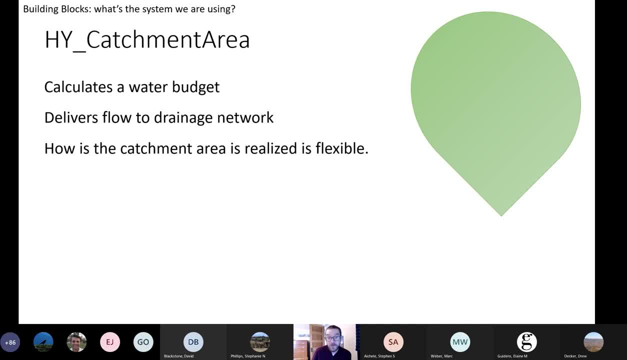 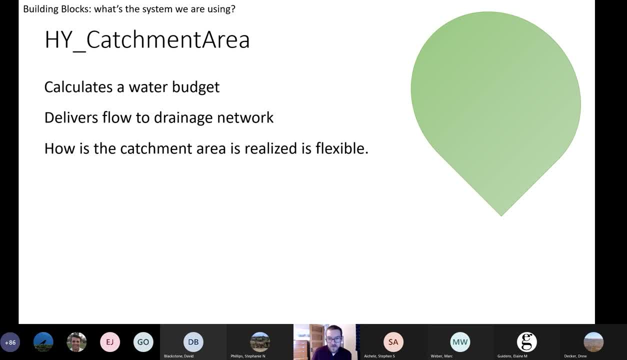 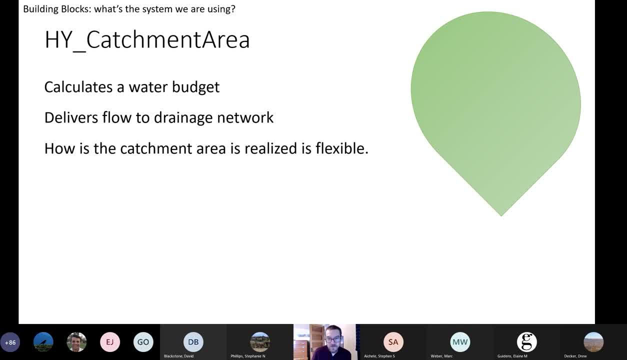 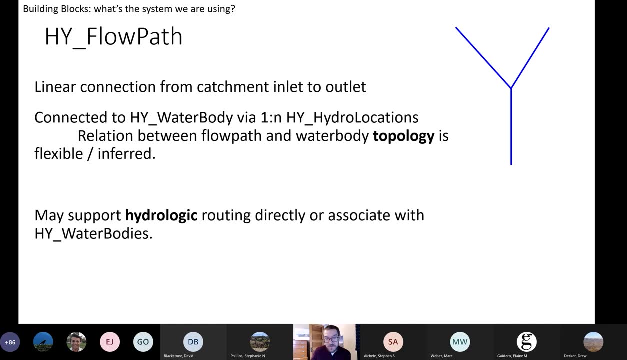 meter grid, do it. If you want to have a catchment area that's represented by one number, do it. They're both catchment areas as far as high features is concerned, And so it gives us a, But then flow path is the next one, And this one's- this one's a little hard to wrap your head. 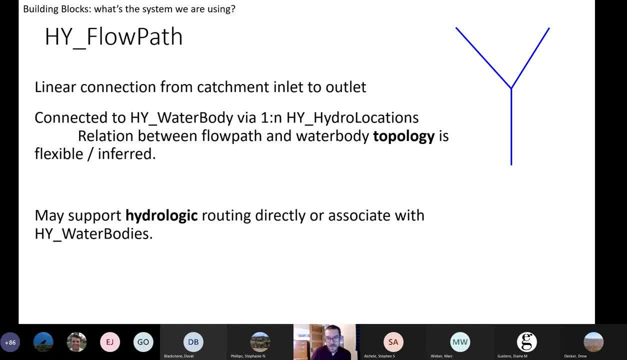 around because it's. it's the linear connection from an inlet to an outlet And it's, but it's not the water body itself. It's. you can think of it as the center line of the main water body that drains a catchment. But for a, for a headwater catchment, there's actually some ambiguity. 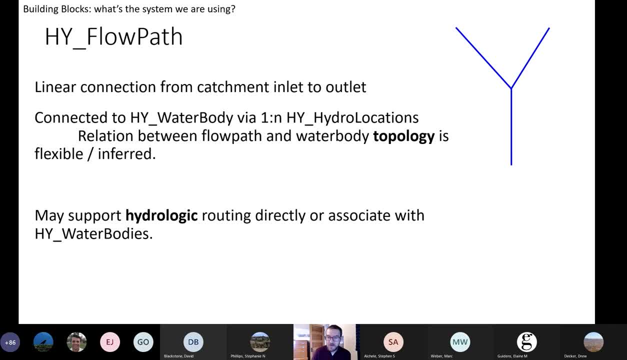 about how you would handle that. The direction I think we have to go is to say the. the idea of a first order catchment is actually that there's a zero order catchment upstream of the onset of flow And the flow path only exists when there is something upstream to. 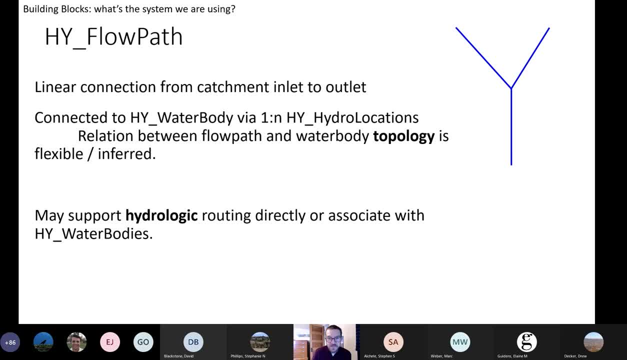 contribute flow, But that's a that's a bit of a side note, but so it's. it's a linear connection from catchment inlet to outlet And it connects of, of, it's connected to a water body via hydro locations, via points that that lie along the water body, And so in that way, 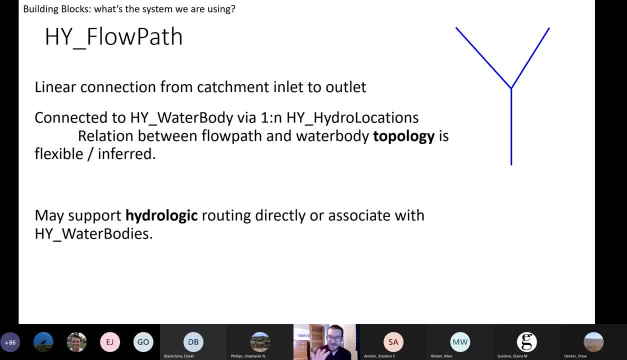 we have a separation of, of concerns between conveyance of flow from the top of a catchment to the bottom and the representation of the water body that actually overlays that conveyance. or or in in classical kind of hydrologic cartography, hydrography, you would overlay a water body. 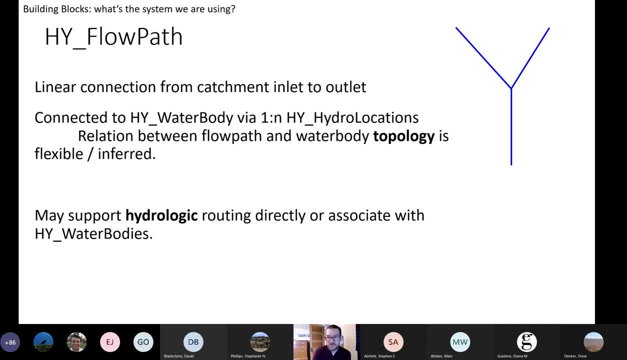 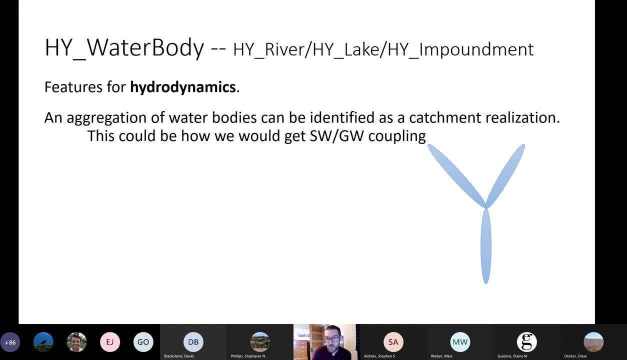 on a flow path and not really visualize the flow flow path because there are no one-dimensional water bodies. You always want to have some overlay. So this may support hydrologic routing, but it would directly associate to water bodies for hydrodynamic routing. So water bodies are. 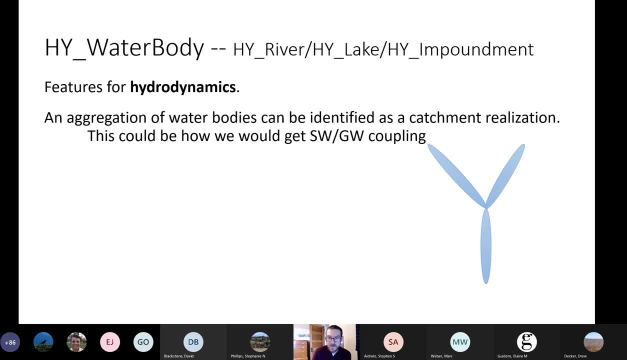 where you would do hydrodynamics or storage And that, and that would be this kind of feature that has two or three dimensions to represent the water itself, And and, and that, when you aggregate all those together, we actually can think of that as a valid 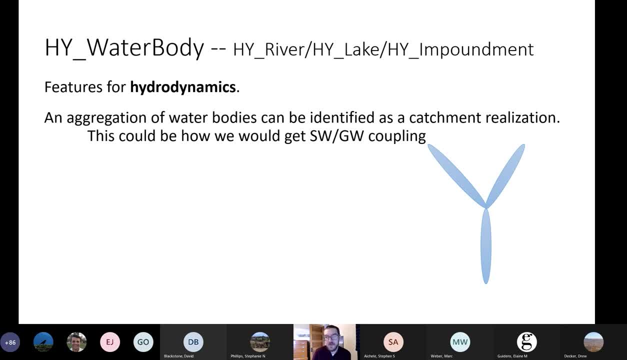 realization or a conceptual representation of the catchment itself, And that's. this is an interesting one, This idea that the, the collection of all the water bodies in a catchment, is in some ways one of the valid cons, partial conceptual representations of that that catchment is. that's. 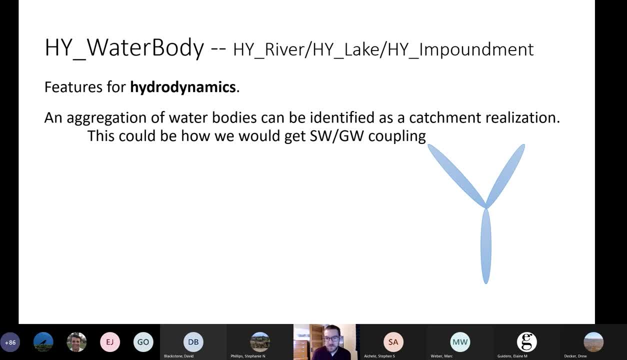 used in a number of data models out there And it's it's something we gloss over. So this is absolutely how we could think about doing surface water. groundwater coupling is having this network of water bodies be the in total set of. 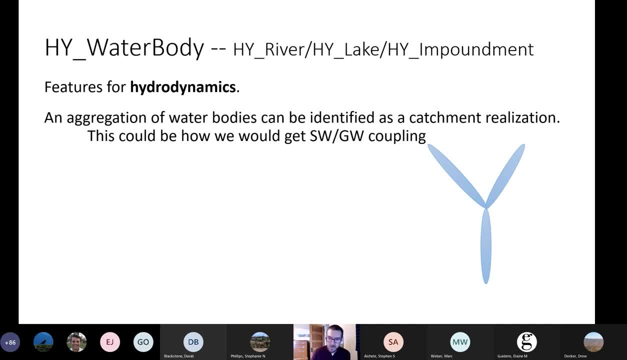 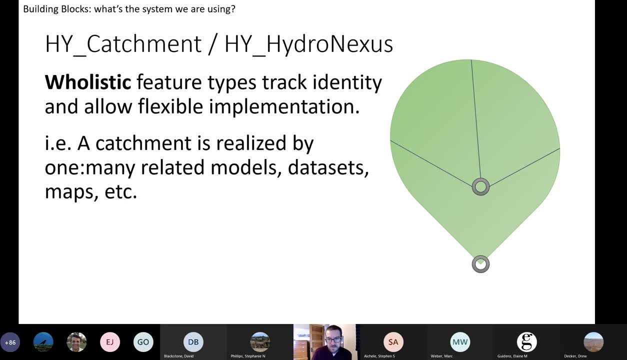 units that have an ongoing relationship with groundwater, But I'll just leave that one there, Okay. So then there's this system of catchments and nexuses that are that are. it's this holistic set of features that low that are related with a common 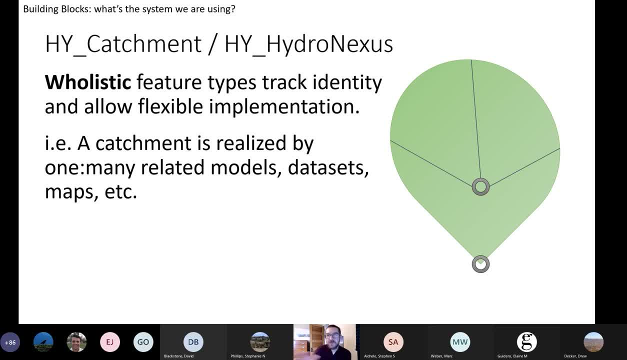 kind of connected system, So so that, regardless of how you represent the catchment, it's downstream catchment is still the same. You know the down, what is downstream of a catchment area, What is downstream of a flow line, What is downstream of the catchments divide around the it's. 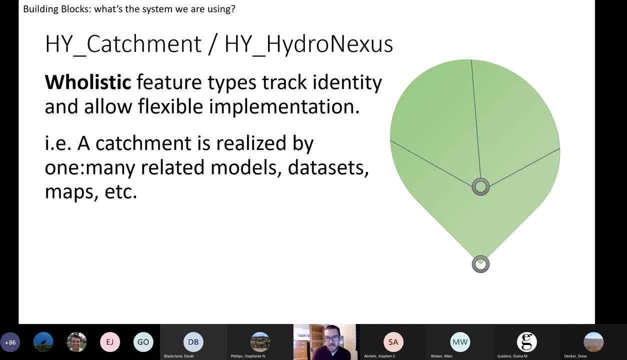 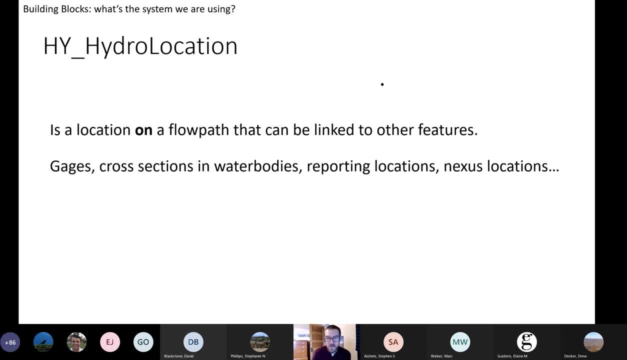 all the same, downstream, upstream connectivity, And so this catchment nexus as a, as a holistic kind of generalization that can be applied to any one of these representations, is really important. And then we've got the, the, the humble hydro location which is used for everything. 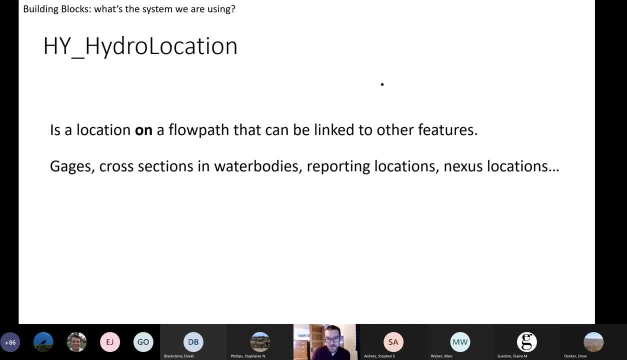 It's a location on a flow path that can be linked to other features, So it gets used for anything and everything, both kind of core, internal things like confluences, or totally secondary, thematic things like landmarks and important locations On the landscape that need to be tied to the, to the, to rivers. 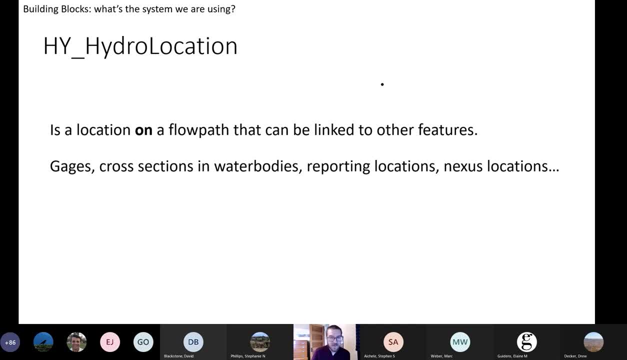 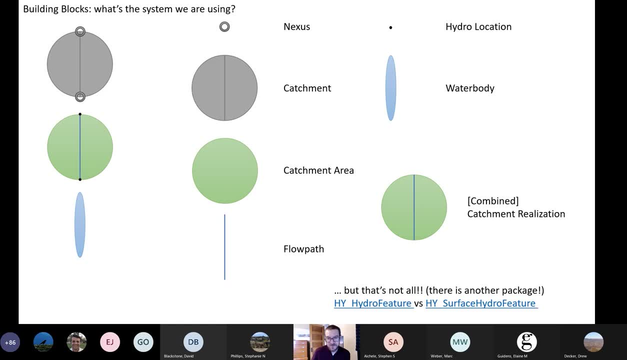 It's the same kind of feature. It's a feature that we ostensibly think is along a flowing body of water, And so those there's. there's a little more in the data model, but that's really the important bits and pieces. I kind of got this into a bit of a graphical representation here, showing 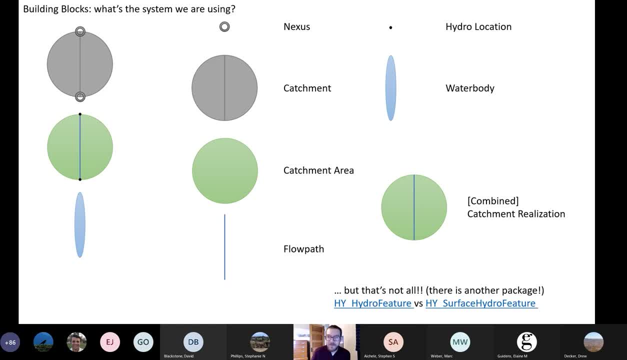 the. rather than putting these things on a map, I find it very useful to think of them more pictorial- pictorially, that's not a word, anyways- in a, in a more cartoon view, right. And if we think of it in this cartoon way, 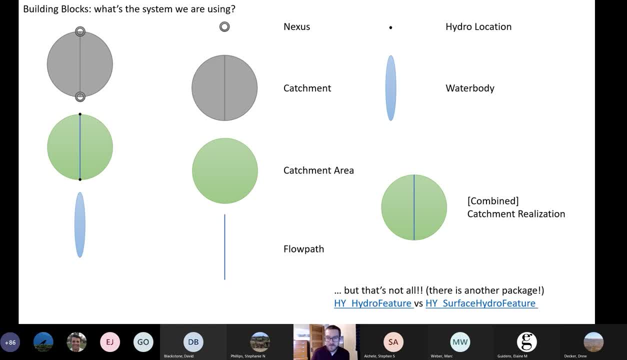 I think it's easier to frame our thoughts in conceptual terms and not jump right to specific examples quite as fast, which can, which can lead to some, I don't know it's. it's hard to. it's hard to make sense of things if you don't have a good general way to to look at and think about it. 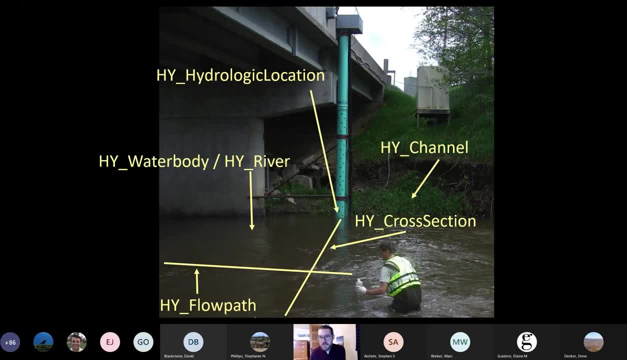 So OK. so coming back to the site that we were looking at before, there's a little more going on. The flow path is actually some linear expression of this river. There's going to be a cross section where we would say the rating curve. 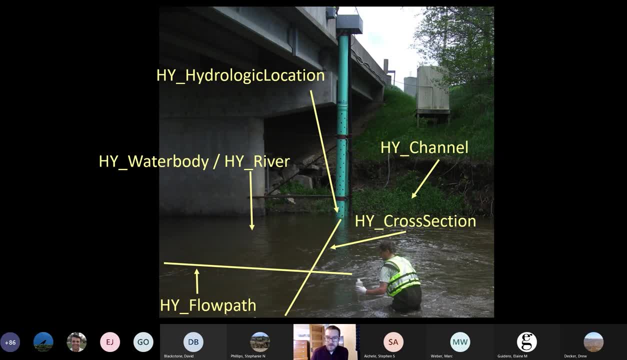 probably for the stage measurement is located There's. there's actually a channel that goes underneath the the water, So there's the, there's kind of the container that this water body is is residing in And and this is all kind of at the same hydrologic look. 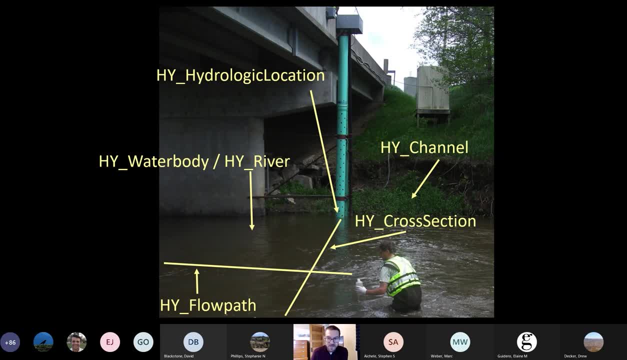 This is all happening ostensibly at the same hydrologic location, which is where the cross section intersects with the flow path, Right, But the hydrometric feature which we would say is that that hydrologic location is off to the side. So so these are all. 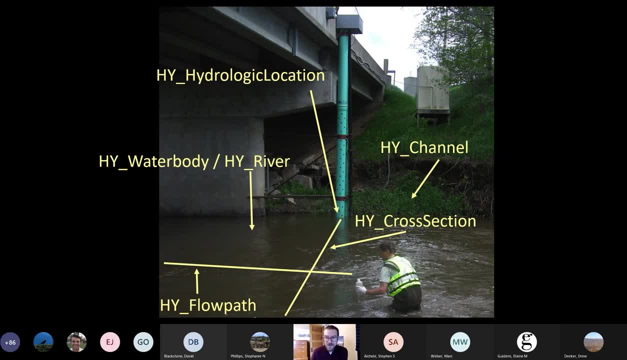 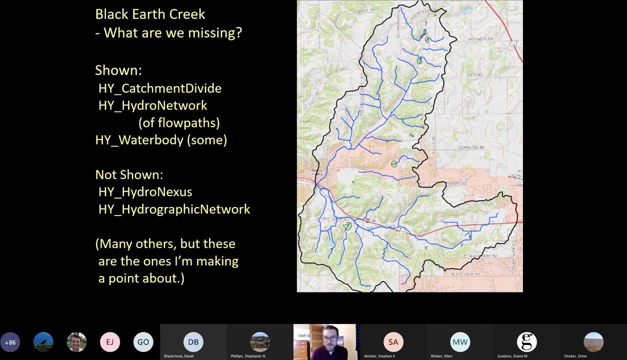 These are all a little a little more distinct features that are involved in this, the scene of of two observations that are ongoing. So there's another example, just to call out a couple of interesting concepts. You know this. this is Black Earth Creek, just just west of Middleton, Wisconsin. 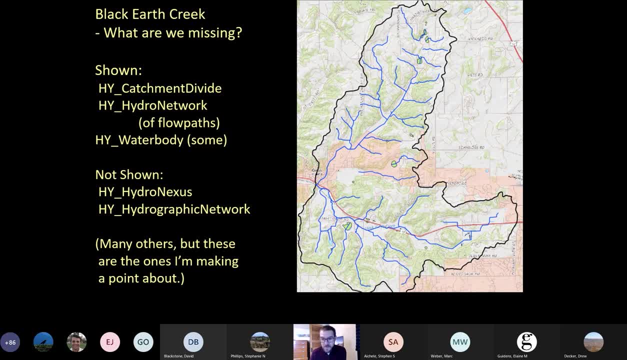 flows, flows out down toward the Wisconsin River And it's a glacial end brain, essentially, or it's a glacial. Yeah, there's there's. there's a lot of glacial material in the valleys And it's fairly steep landscape. 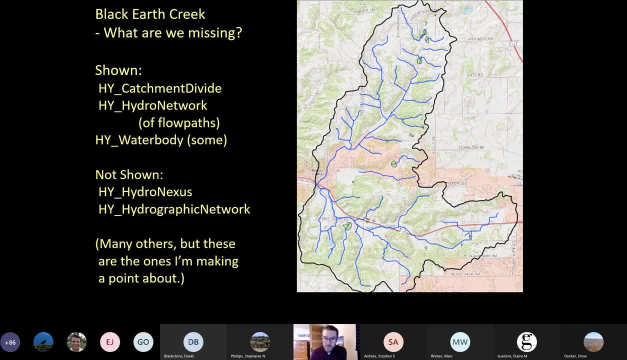 And so so there's a lot of gravel in the valleys And what you see here, these, these flow lines that stop, these flow lines that stop. there's a couple here. I think my mouse let me- Yeah, you should see my cursor. 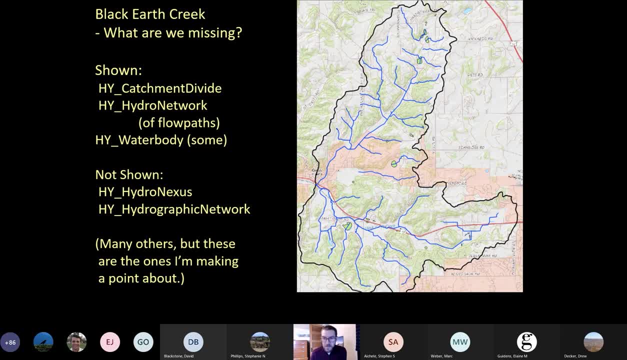 There's a couple here and there's a few up here. These actually just flow into gravel swales. that if you were to track the soil moisture the, the water clearly flows to the river And the fact that there's surface disconnections really from a hydrologic point of view, is not correct. 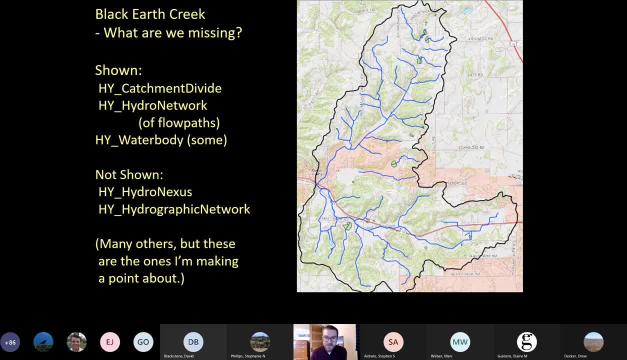 These, these flow in a surficial sediment, And when it rains real hard there is overland flow. There's just not necessarily evidence of it when you look on the landscape. So so that's just something to point out. This, this kind of indeterminate surface connector thing, is something that hit. 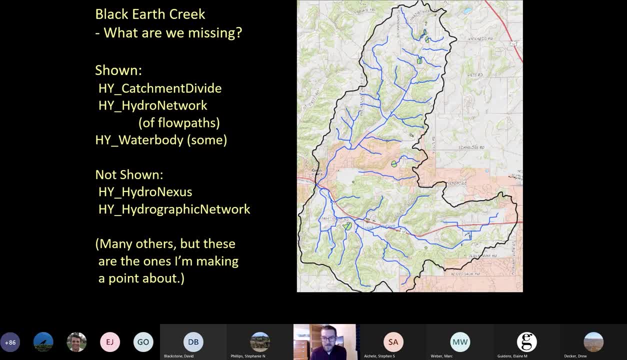 the 24 K and finer resolution of hydrop hydrography really needs to be thought through and included, And so so that's that's the systematic thing we're missing, But so so shown here we have the black and the catchment divide. 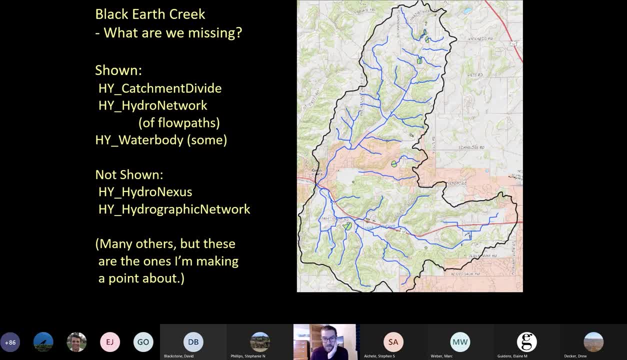 The network of flow paths is the blue the, the water bodies. There are some of them. There are these? not sure that these are technically water bodies, but they're. they are sometimes ponds essentially that I think are mostly just wet wetlands kind of thing. 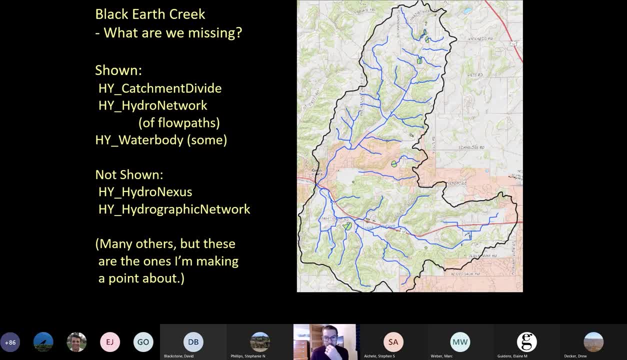 And not shown here is is the, the hydro nexus, or the hydrographic network, And I'll get to what I mean by the hydrographic network On the next slide, The, the hydro. So the hydrographic network is supposed to be the network of water bodies. 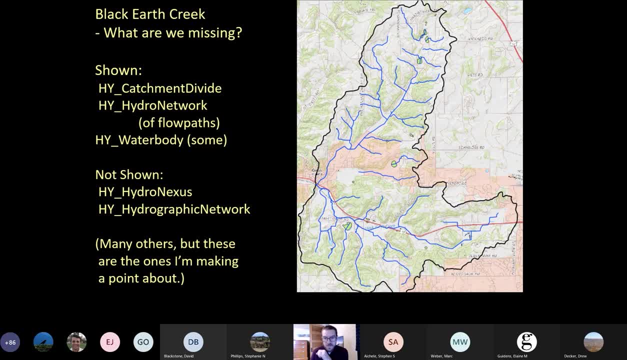 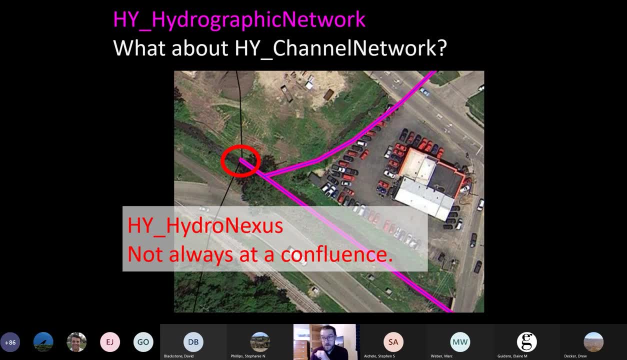 And so what we're showing on the screen here is one dimensional representations of the hydrographic network that are that are truly one dimensional. So they're flow paths. They don't have any width. They're not representing any water. They're, they're representing a of 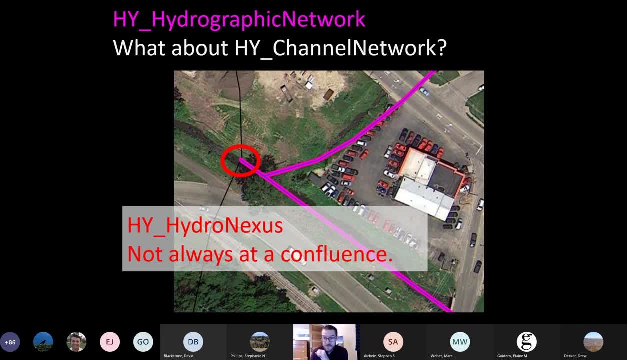 infinitely narrow Path across across the landscape. that happens to coincide with where water might be, But if we zoom. So this was. I made this graphic a while ago where the slide is hidden right now. But that pink line is roughly the nominal pen width of a 24 K map. 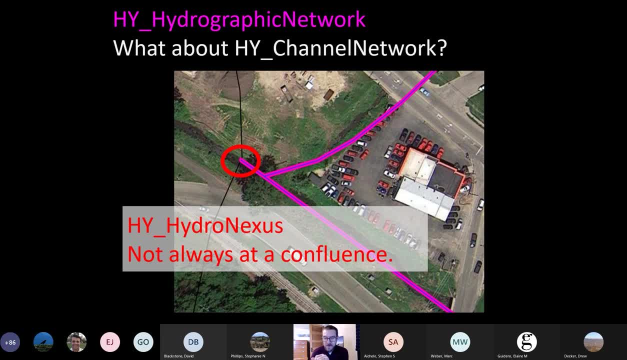 blue line And so so, if you track with what I mean there, at the 24 K scale, a blue line has some nominal width and that pink polygon is that nominal width. That's what you would really want. When you said hydrographic network, you would want to say, well, the river is. 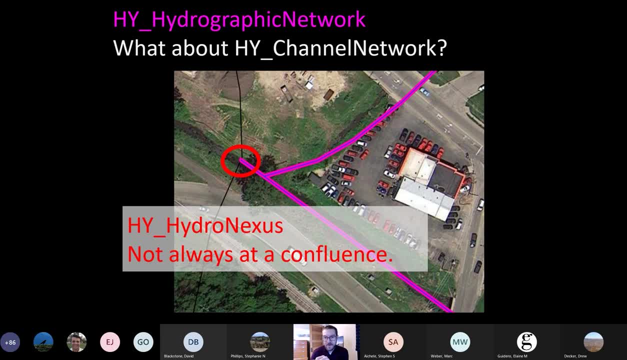 roughly this wide. So we're going to put a, put a polygon around how wide it is at a at a scale that are at the actual visualization scale. But we don't do that with one dimensional hydrography, We just have the blue line. 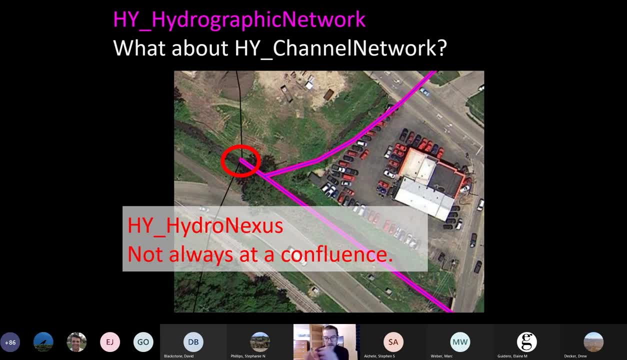 And we have a pen width that we choose for that blue line at a given scale And that typically works out. But this separation of one dimensional feature and two dimensional water body representation is really important as we get into finer and finer resolution representations and expect to use this data at multiple scales, which we do right. 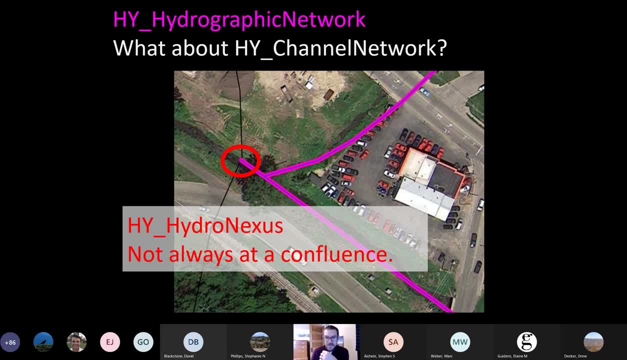 And another thing to point out here is that this nexus thing isn't always at a confluence. So this data set that I chopped out, I believe either at a WBD outlet or a catchment boundary, The confluence is just upstream of the edge of the. 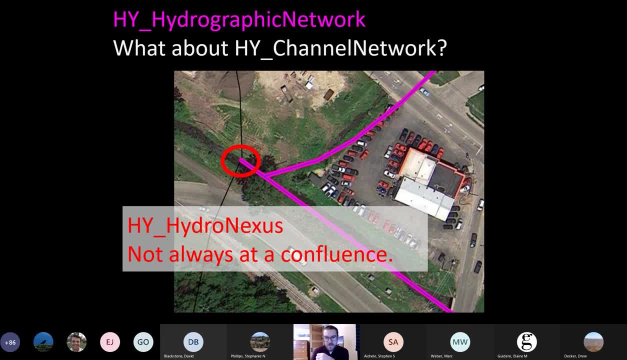 the drainage basin, the edge of this watershed, And so we would say that the nexus for this black catchment divide is actually here, not at the confluence. And yes, logically, there's a nexus here, because there is a watershed for this flow line and this flow line. 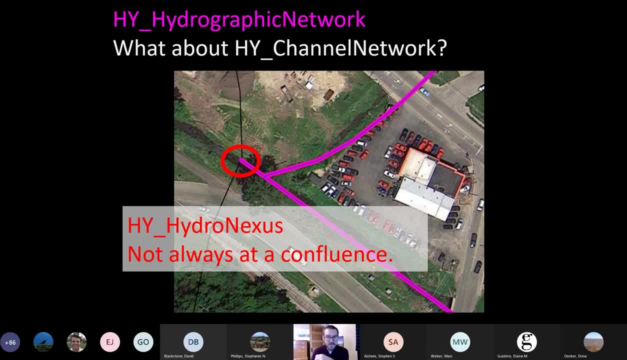 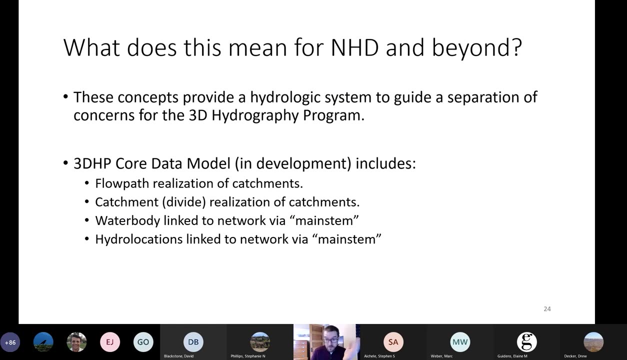 But just the this: this idea of a nexus is not necessarily only at confluences. It's something that can exist at any boundary between two catchments or two, two watersheds. OK, so what does this all mean for NHD and beyond this 3D? 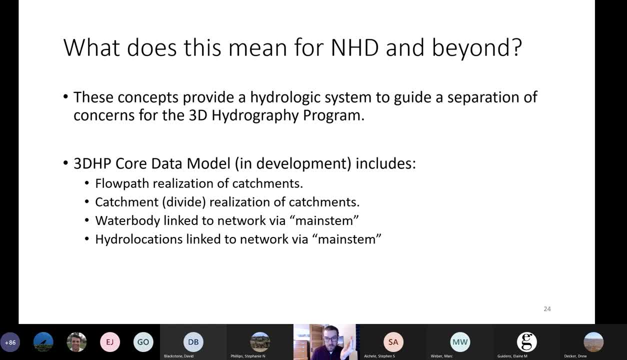 hydrography program, work that's ongoing. I kind of. I think I've alluded to a lot of this, but you know the concepts here are providing us a system that guides this separation of concerns to make sure that what we're doing is as. 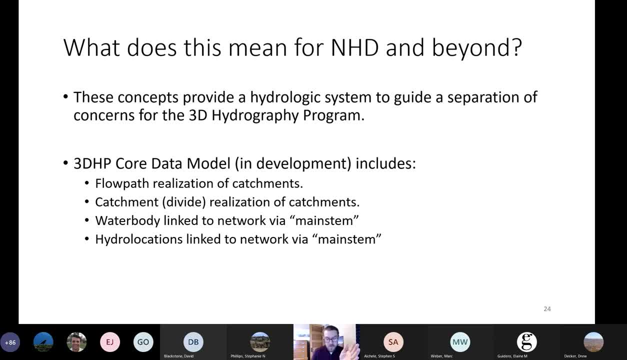 as simple as possible, but no simpler right. That's the, that's the trope, That's what we're going for. How can we distill this down to component parts that have one job and they all fit together as a really coherent, really cohesive system? 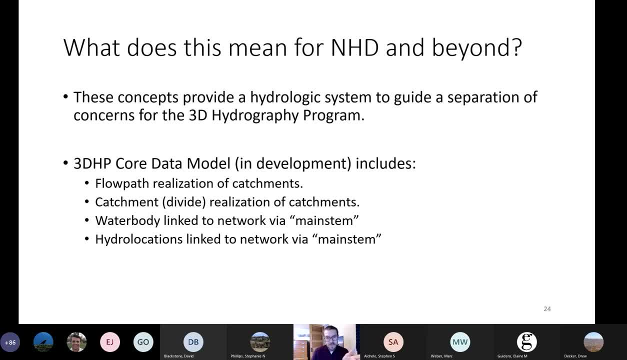 Right, And so we're using all these techniques and these tools to get us there. And then you know the the kind of the testing tests that we're doing today are really going to be a bit different and concrete And concretely, what this is turning into in this 3D hydrography program. 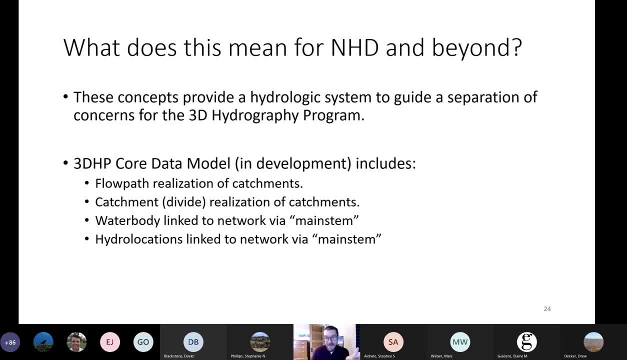 data modeling exercise that we're undertaking right now is that we'll? we'll have these features I've been talking about. There will be a kind of flow path realization of catchments that will probably be made up of multiple flow lines, quite similar to well. 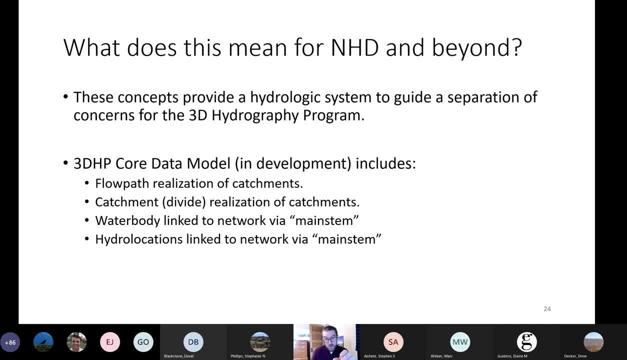 a flow line going through a field that then goes into a culvert. you wouldn't necessarily draw a catchment around the culvert, but you may need to break that flow line into two pieces: The union of those two or the aggregation of those two flow lines: the one in the field and 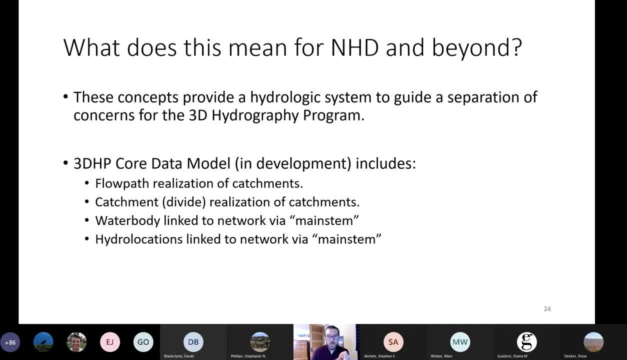 the one going through a culvert is one flow path which would have one catchment, one catchment divide ostensibly. So that distinction of flow path is one that's going to be needed, especially now that we're into this EDH, you know, elevation drive, hydrography, super high resolution, kind of. 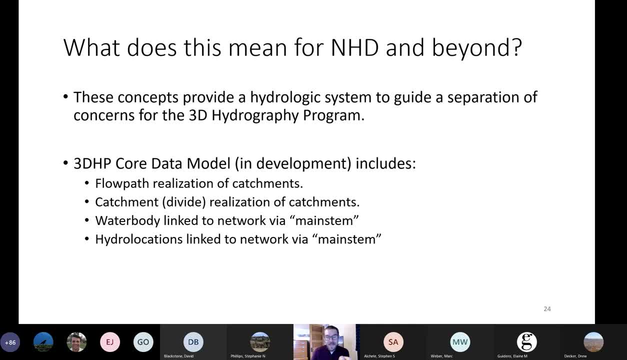 granular features. Having the ability to aggregate features into catchments that are of some reasonable size is really important, and that's where this flow path thing comes in. And then, so catchment divides will be one of the things that we're going to need to do, So that's one of the things that we're. 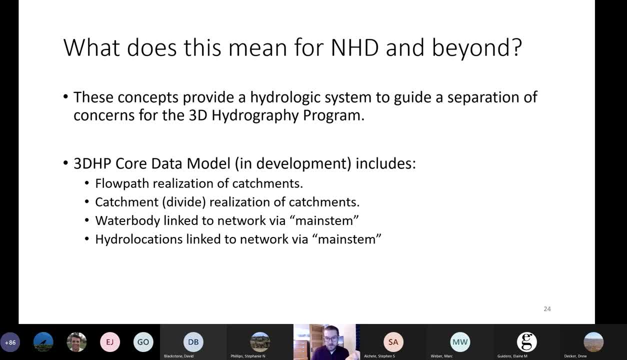 going to need to do. The other will be the other main kind of conceptual realization of a catchment that's included and that you know. having a catchment for every incremental flow path allows you to do drainage area, which is really useful, allows you to link the landscape to. 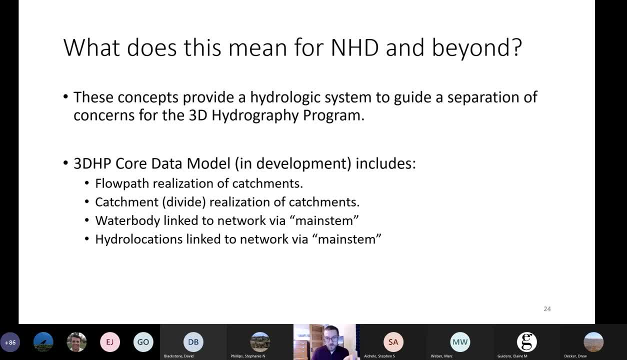 your network in a concrete way. That's super duper key. And getting that core to the process, not as a post-process as has been done with NHDPlus, is super duper. important Water bodies linked to the network via this concept of main stem, which I'll get into. 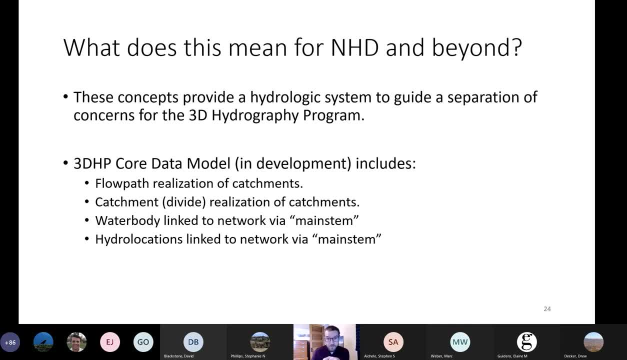 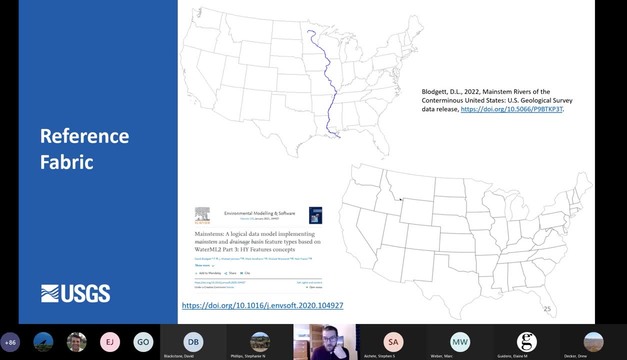 realizing I'm going to move along here- Hydrolocations linked to the network, also via main stem, and this main stem thing is what I'm going to talk about next. So, main stem, I've been working on this national reference fabric thing, largely in service of the 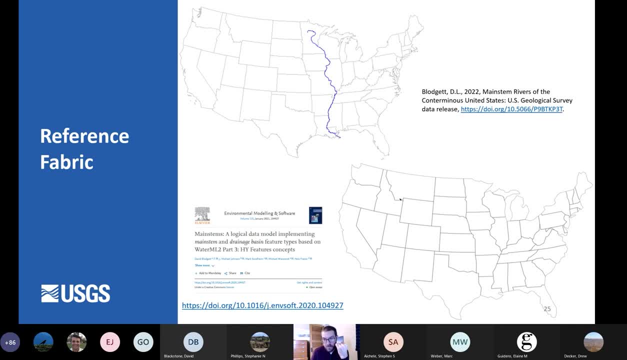 national water census For a number of years now. The original work I did on this finally got published in 2020, but this work really started back in like 2016 or so And hopefully these animations are working for you. This is one is showing the major main stem rivers, kind of animating in from most dominant. 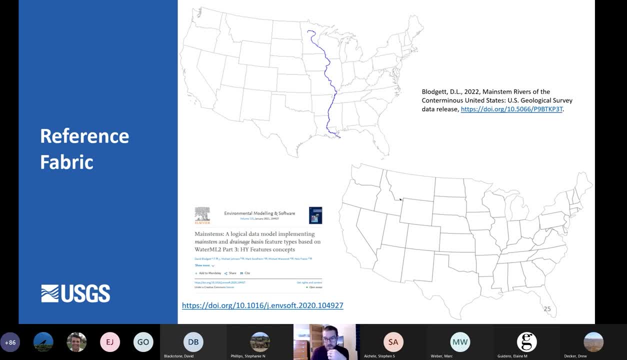 or largest to smallest. And then this other one is the watershed founder dataset, animating from headwaters to outlet, where all the outlets kind of coincide at the ocean right, And what I was trying to do with this work was figure out how to estimate stream flow for 12 digit. 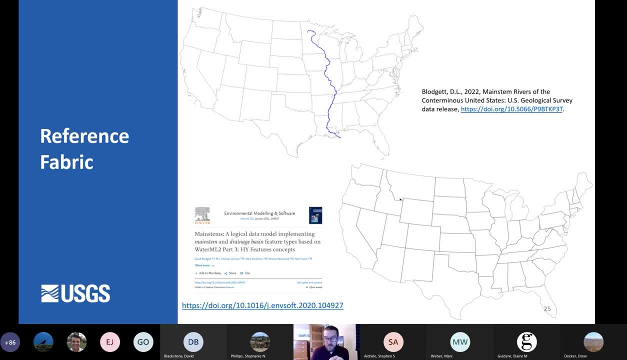 hydrologic unit code watersheds, which is really hard because the watershed boundary dataset is not tied to the river network, at least not in an explicit way, And establishing that correspondence between NHD rivers and WBD units turned out to be a great problem to solve, but turned out to be a 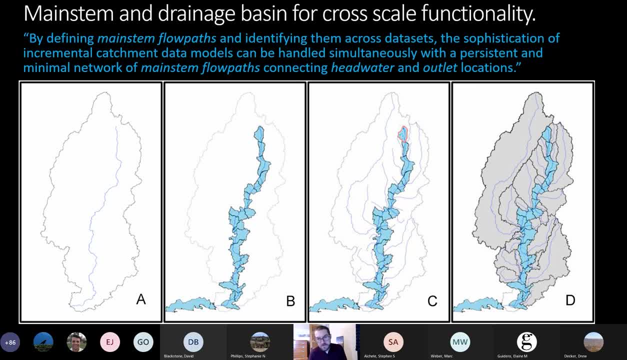 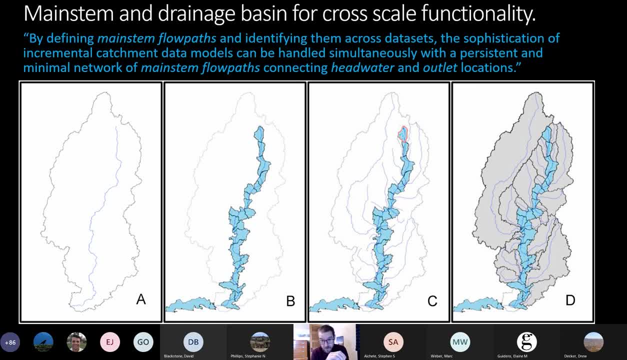 And so this quote from the kind of original mainstems paper. By defining mainstem flow paths and identifying them across datasets, the sophistication of incremental catchment data models can be handled simultaneously with a persistent and minimal network of mainstem flow paths connecting headwater and outlet locations. 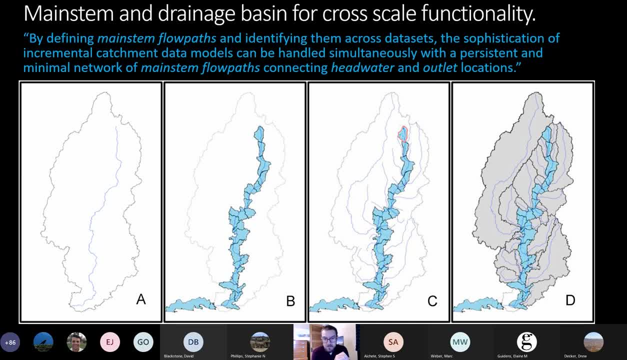 So this persistent and minimal is really important. We're trying to minimize the number of features we need, So this persistent and minimal is really important. We're trying to minimize the number of features we need, to maintain in a persistent way, um, but maximize the functionality we can get out of them, right. 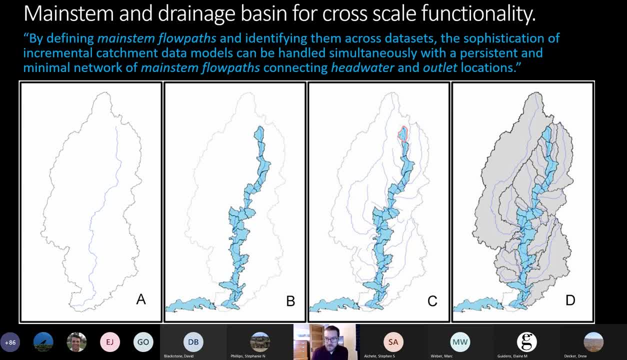 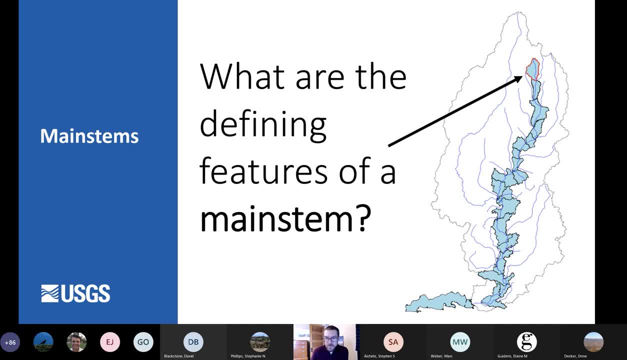 and that. so that's the real, the real kind of functional purpose and core goal of this main stems work. so what's what's defined? what's defining a main stem? um, first, it's a headwater, some headwater location, and i made a side comment about headwaters and zero order streams and that. 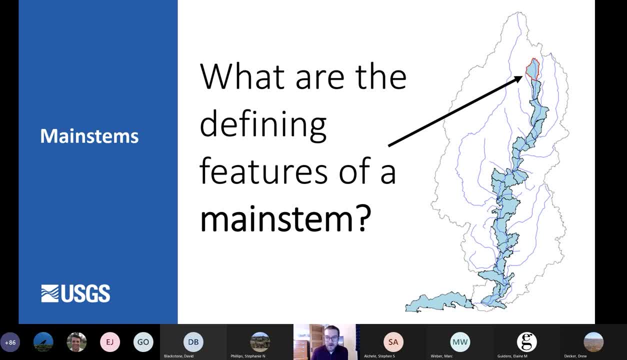 and the reason i have put a lot of thought into that is that the headwater is really the, the key seed for a main stem, because the rest of the main stem is a path to some outlet right, and so this pair headwater outlet path, or this pair of headwater outlet, 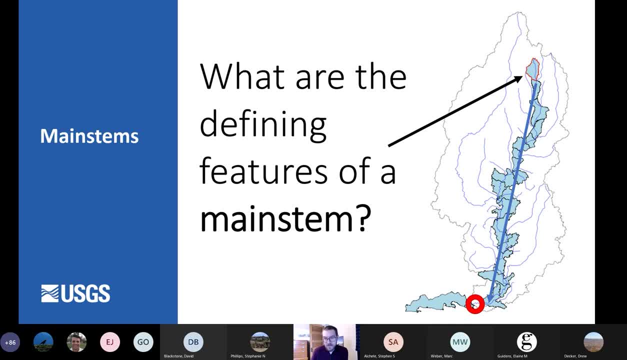 and the path that connects them, the primary downstream path that connects them. this is what we expect to be persistent through time in the the future kind of 3dhp- 3dhp program data sets. we'll have an identifier that says from this headwater identifier. 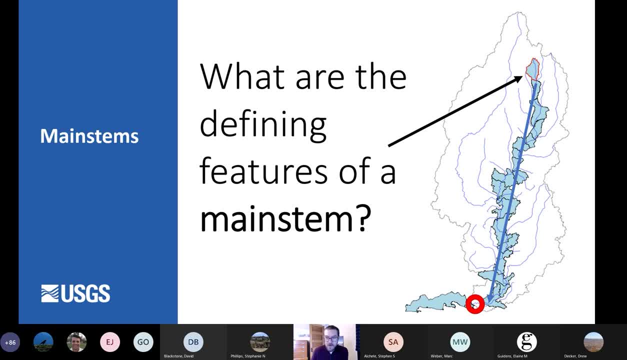 to this outlet identifier. there is a path and we know that that path is the same, that headwater general, headwater area, general outlet location are the same as the data set evolves through time. and by maintaining persistence on that level of identifier and network connectivity, we have the opportunity to accurately um conflate. 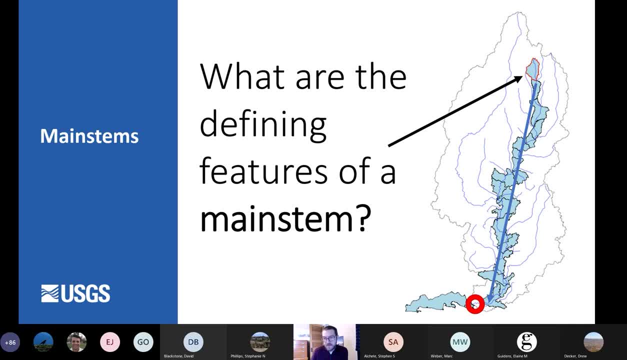 and migrate and and use data in a way that's hydrologically accurate and hydrologically representative- um, as long as we're tied to the same main stem anyways, and so carrying that main stem identifier around, using that as our persistent identifier, is going to be going to be really key. 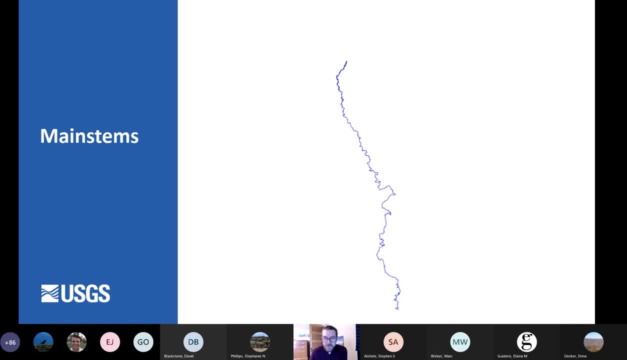 so, then, what this turns into- and this is pretty intuitive- is is it's the tree that connects the landscape, and if you have a set of drainage basins, um, these are, these are wbd units that correspond to a collection of i think this is 100k nhd in this case, but this works for any network. 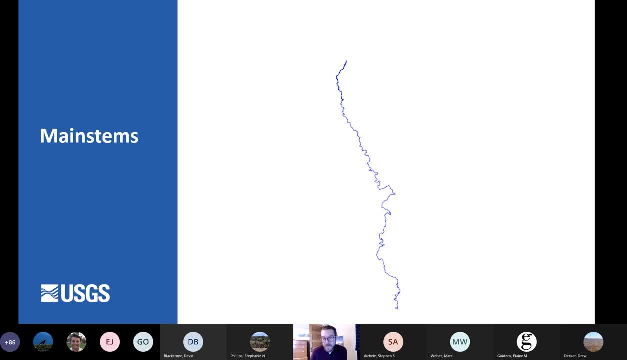 if you have the incremental drainage, drainage areas, catchments, that correspond to the, the components of a main stem, as you densify that main stem network, eventually you cover the whole landscape and this, this is really the the kind of gee whiz right. this gives you this system. 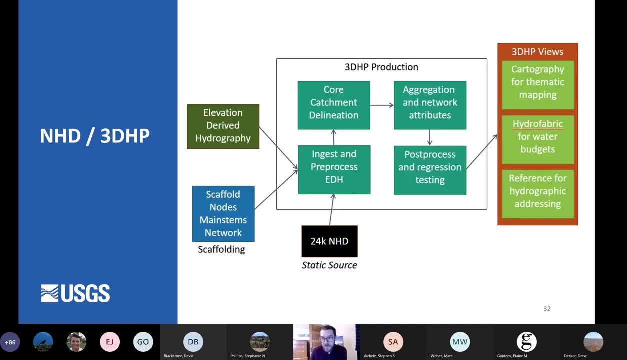 that completely covers the landscape. all right, so let's talk a little bit about the 3d hydra program, um, and where this is heading um. so this is a- this is a very basic graphic that's illustrating where we see this going right now, and this is a work in progress. um, this, this diagram, isn't saying: 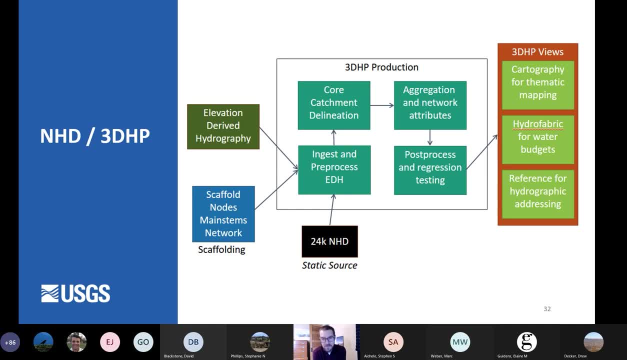 more than we pretty much know right now, but i do expect aspects of this diagram to evolve over time, so just subject to change. caveats all over the place, um, but in essence, what we're imagining is that there will be a core production process that takes elevation-derived hydrography. 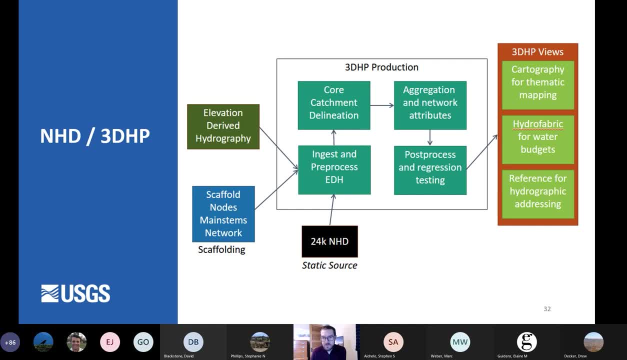 delineates catchments for some set of um aggregate flow paths um. so exactly the size and logic used to to decide what we will delineate catchments around has not been established yet, but that's a piece of the design process right now um taking those catchments. 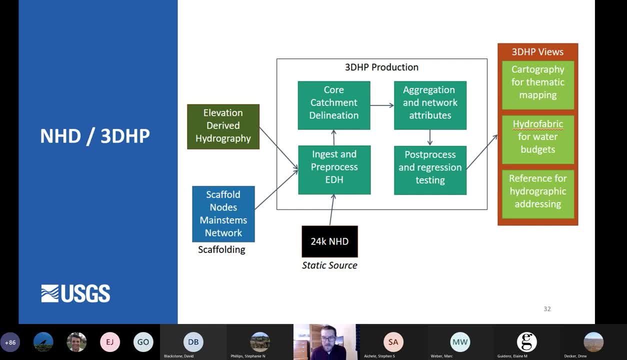 aggregating them to drainage units of some kind akin to the wbd, and building network attributes akin to what you have from nhd, plus running some kind of post processing and regression testing to you know, clean the data, double check, everything is the way we expect it to be, etc. etc. and then set. 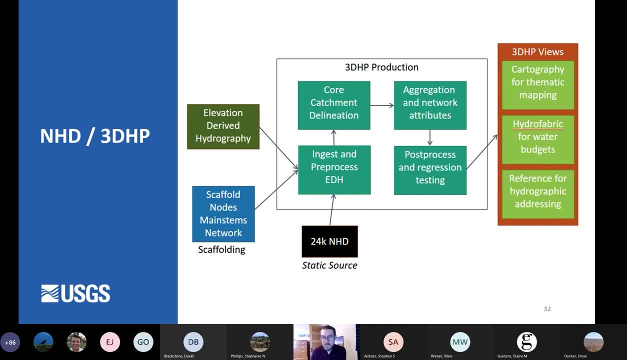 up a set of views. that would be the way that people actually interact with this data set, where there's a set of views that are appropriate to certain applications, um, and and so we have this kind of common set of information that we can build by bringing in elevation-derived hydrography. 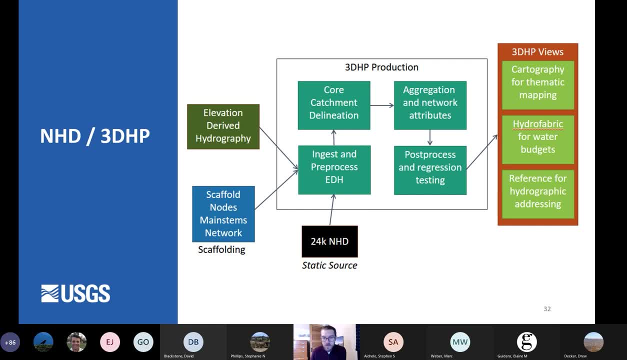 historical hydrography, um, a set of pre-existing persistent kind of nodes and main stem river identifiers, piping all that through a production process and then delivering that out to something that meets particular people's applications and needs. and so this cartography, this cartography is going to look and feel very much like the existing nhd, the reference for hydrographic. 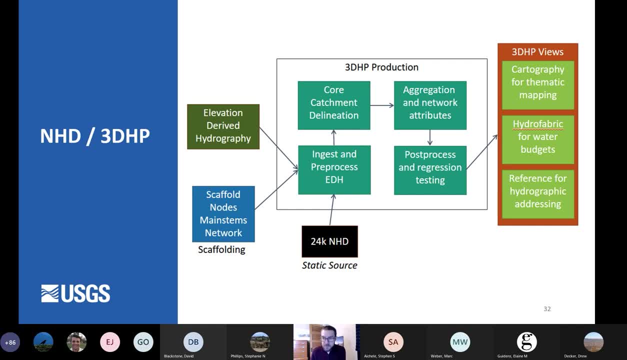 addressing will give people um a bridge from existing reach code and measure events and linear referencing to this main stem based um kind of scheme for hydrographic addressing. and then there'll be a hydra hydra fabric for water budgets that's going to function and look and feel an. 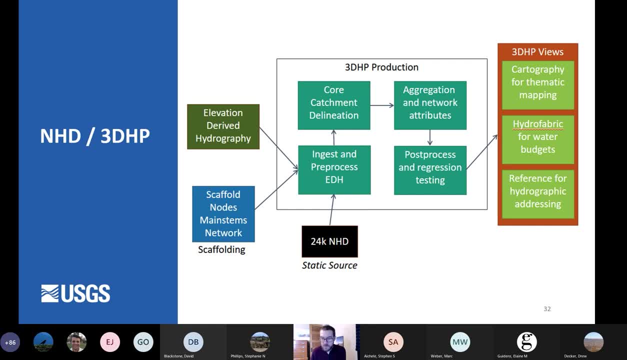 awful lot like nhd plus and and kind of meet the modelers where they are or meet the people that need to do hydrologic analysis where they are. so those are the three views that are really in scope right now, but there's a list of another. 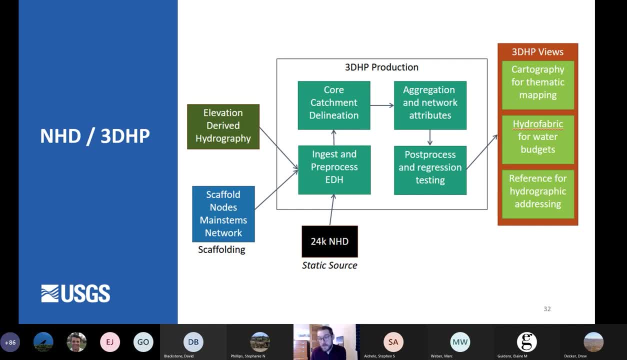 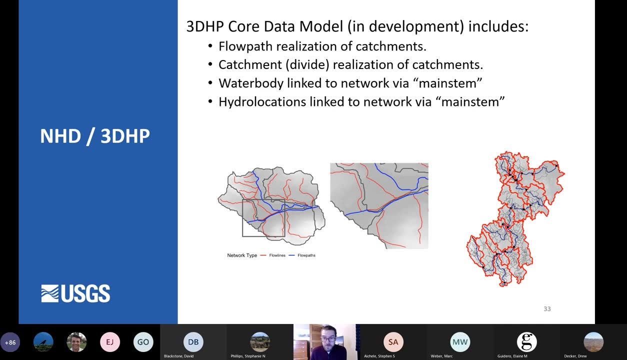 half dozen to dozen um. that's on the horizon and and so adding additional conceptual or or concrete views of this to meet particular people's needs is absolutely on the on the roadmap. so that's pretty much it, um. you know, with the, the, the, this, this data model in includes these feature types that i mentioned earlier. um. 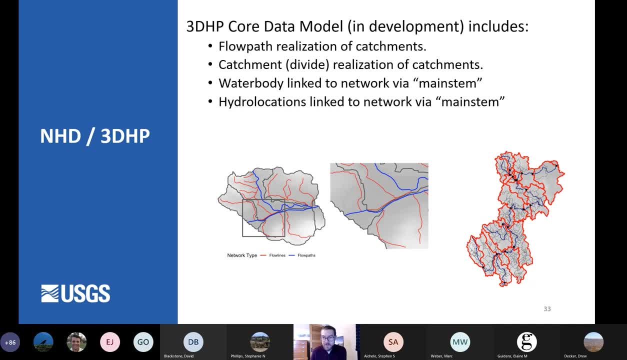 so flow paths. 1d representations of the: the path from inlet to outlet. catchment divides that encompass the, the, the area within a catchment, the, the set of water bodies that we can link to flow lines and and link to main stems for kind of a persistent 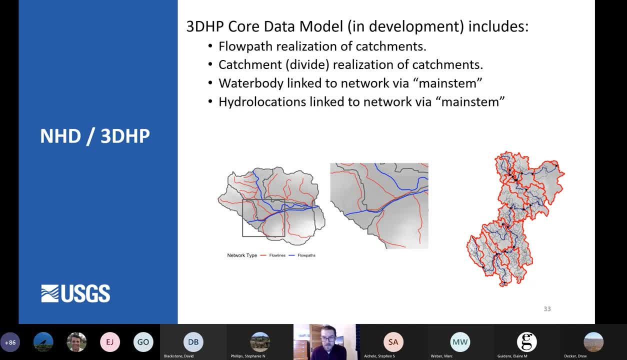 a persistence layer that gives us that hydrologic kind of continuity, and then hydro locations, and there's a whole slew of different types of hydro locations that would be linked into the network also via that main stem and um, i think that's what i have, okay, well, thank you again. very much, david.